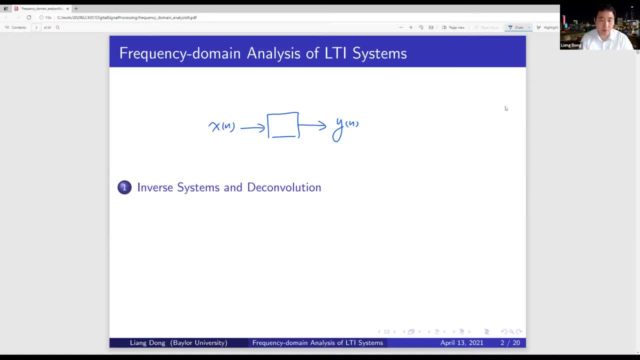 is the original signal x, For example, that can be a communication channel, So the channel itself is any transmission media And we don't know that And what we have here is observed. the signal y- Now y can be, can have. 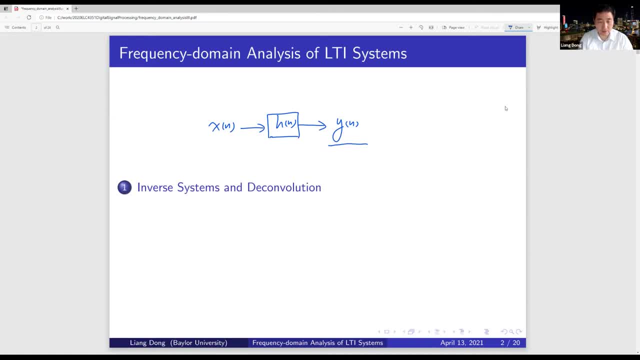 a lot of those, this filter, this filter edge effect, And it's corrupted. either it's corrupted or distorted version of the original signal x And we want to recover the original signal x in- let me call it, x hat estimator of x. So we have another filter here called edge prime. 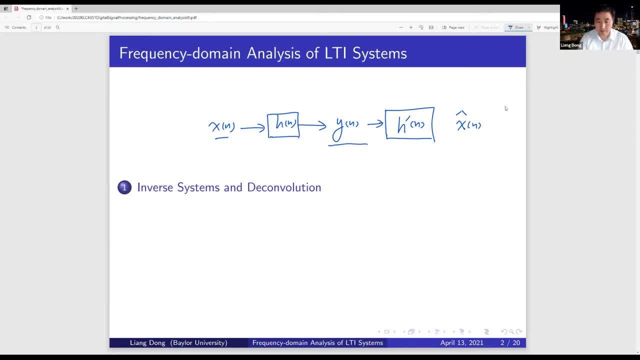 This edge prime is an inverter In time domain. we can think that as a deconvolution, we're trying to find x convolve with y equal to x convolve with edge equal to y. But we have y And if we have edge, if we know some edge edge, I want to deconvolve and find the original signal x. 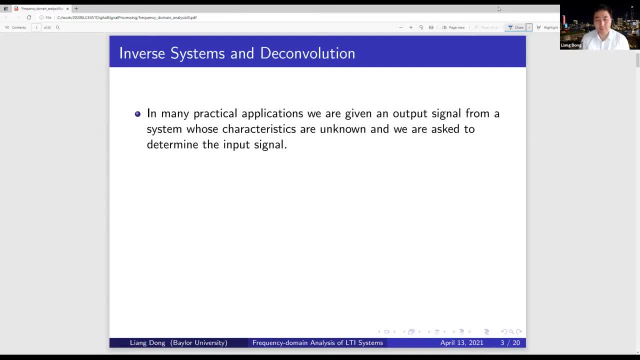 In many practical applications we are given an output signal from a system whose characteristics are unknown And we are asked to determine the input signal And we find something from the, from the input signal Input signal is is not. no, it's not observable directly. 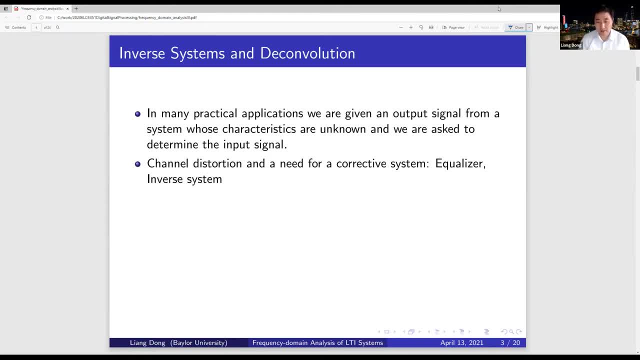 Channel distortion and a need for corrective system. So this is an inverse system. Now, what is channel distortion? Channel distortion, as I said- let me use this In in, for example, communication system- is I have the signal coming here. 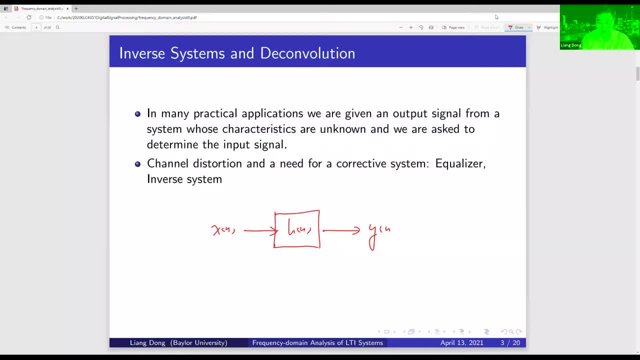 Go through a channel and then I have to receive six signal. This is the received signal, Now the channel, for example. the channel is very simple. We have a wireless communication channel for, for example, And then the signal coming in because it go through the media, media- is the, the free space propagation. 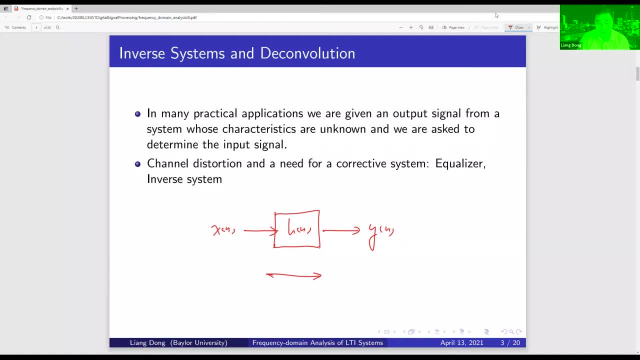 So it can have impinging waveform. It may have another reflected waveform from the ground, from other buildings, So these can be used in space. these are this one and this one. those are the multi-path. this multi-path has a delay effect, so the channel itself is in a delay effect. so we have looking to this h in in the time domain. 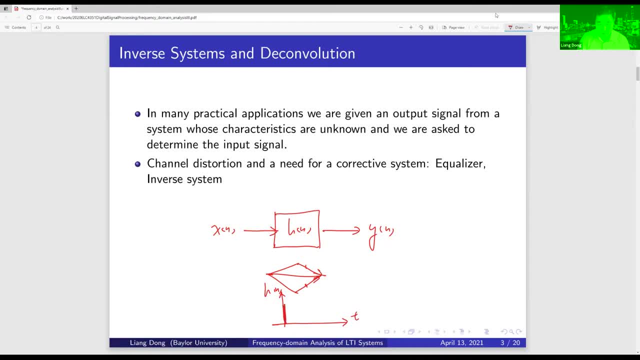 so we got an impulse here, which is the first impinging wave. then we have some delay effect. these are due to those two multi-path. so if i have in the time domain those delay effects, so i have not only h 0 but i have h 1, for instance, i have h 3, for example, h 2 is 0 here. 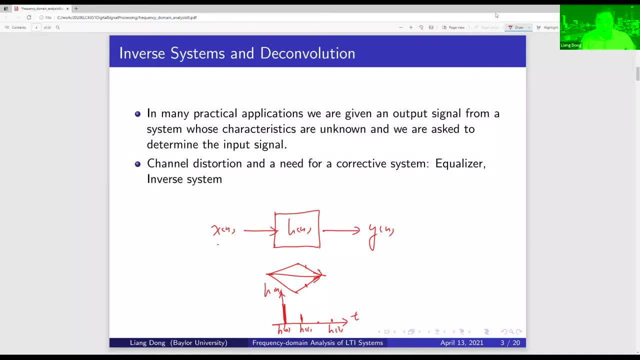 the signal x, n will go through a finite impulse response. right, this is a finite impulse response. the impulse is not just a delta, but it has some other, some other parts here, with a, with a support that is expand just one time, instant. then i have the received signal at y. 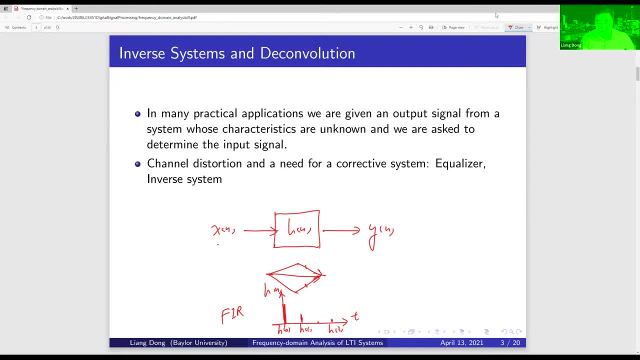 if this is FIR system, look like that. it's a delayed, it's a delayed element here. what will that give us in the frequency domain? in the frequency domain, that will give us some frequency selectivity. so in the frequency domain, roughly speaking, f, h, omega instead of being flat. 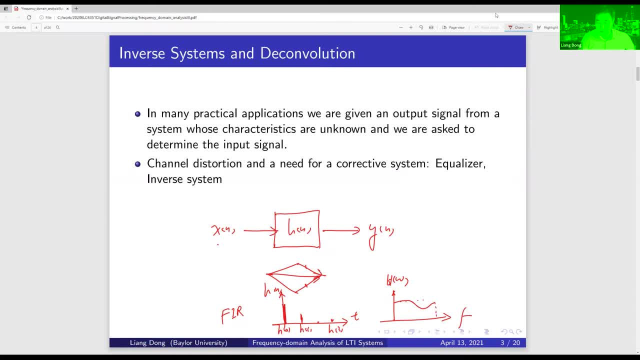 it will have some effect, maybe like this for, for example: so this is the frequency selectivity, so some frequency will be emphasized, some frequency component will be de-emphasized, and that is a frequency filter filtering the input signal x. and then what we want is: i want to have an equalizer. now, this equalizer, i want to multiply. 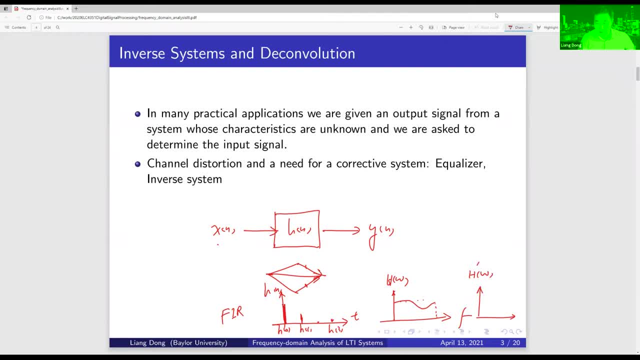 for example, let me call this h prime omega and the effect is- let me just draw this way- the effect is h prime multiply by h. then i will have a flat line across all frequency. and that's what an inverse system will do. because it does that, we call that, we give a name called equalizer, we equalize the frequency. 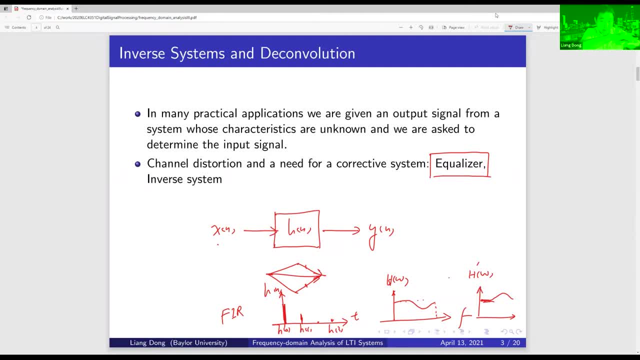 component, make every component of the frequency part equal. it's evenly, evenly distributed. so that is an equalizer, or we have many good use of an equalizer and we have many different ways we can deal with that. okay, so in the inverse system- the inverse system is a corrective system that has a frequency response. 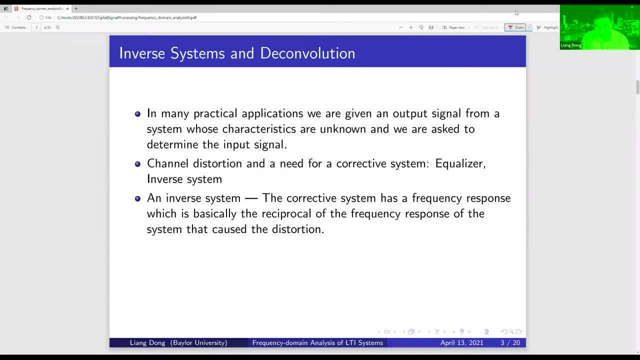 which is basically the reciprocal of the frequency response of the system that caused its distortion, like we seen in the on the previous page, deconvolution. deconvolution is the inverse system operation that takes yn and recover xn, so the effect in time domain is a deconvolution. 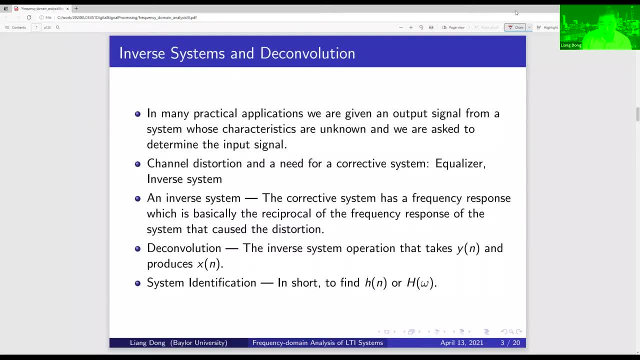 so the effect in time domain is a deconvolution. the system identification is is another kind of deconvolution. now this deconvolution here is: we know y in. i also estimate a system. i want to find what is my input x, what is input x. so we do a deconvolution. 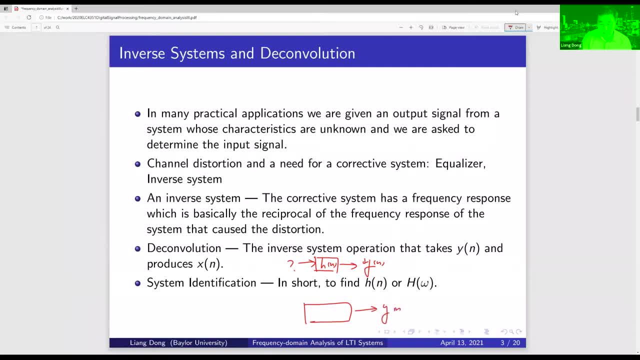 system identification is that if i know why, i observe why i know what is the signal to the system, to find what that system is. That is we call the system identification. We have done that before. We solving for a difference equation is that we know the input X, we observe the output Y. 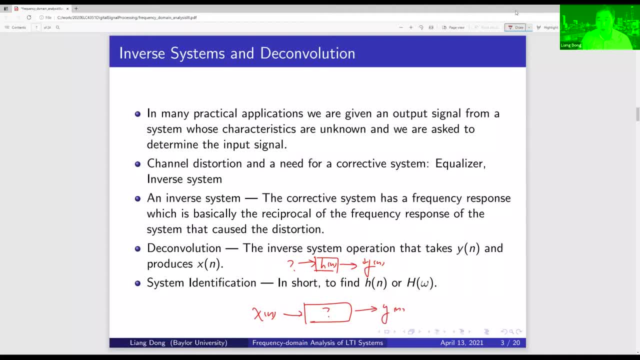 and then we putting everything into a difference equation, Then we solving, we solve for this difference equation. find out what HN equals to. That is system identification. System identification- we can go ahead and find a little HN in time domain. 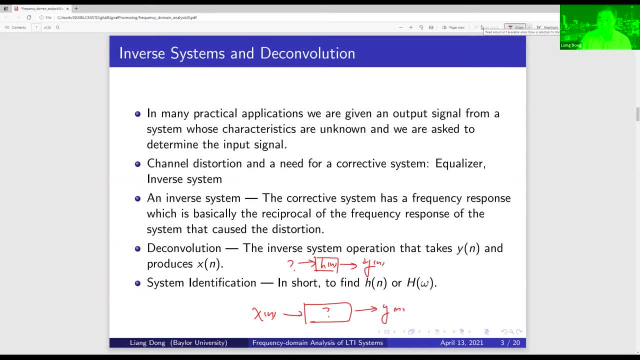 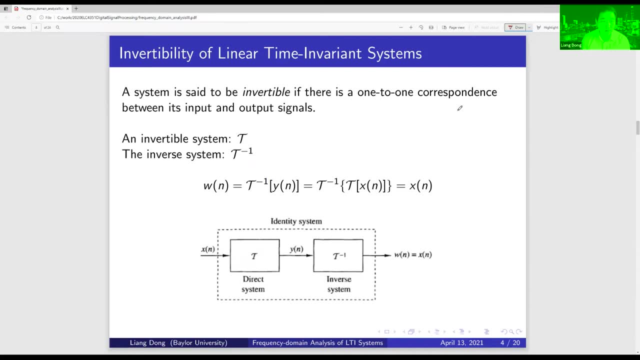 or we can find the capital H, omega in the frequency domain. Either way, we can find the system, We can identify the system. A system is said to be invertible if there is a one-to-one correspondence between its input and output signals. 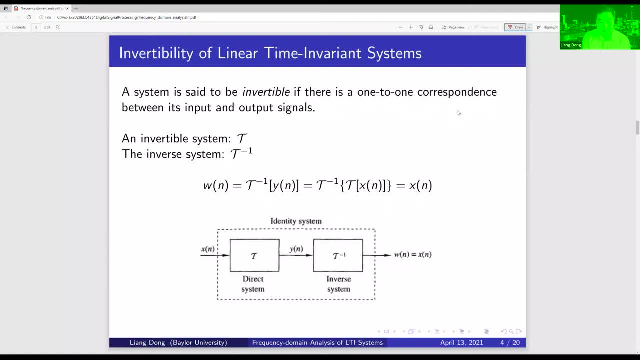 So an invertible system represent as a linear operator T, Then its inverse system is T to the power negative one, And it's inverse, And we want to emphasize that- because in frequency domain T multiplied by its inverse system, which should give us identity. 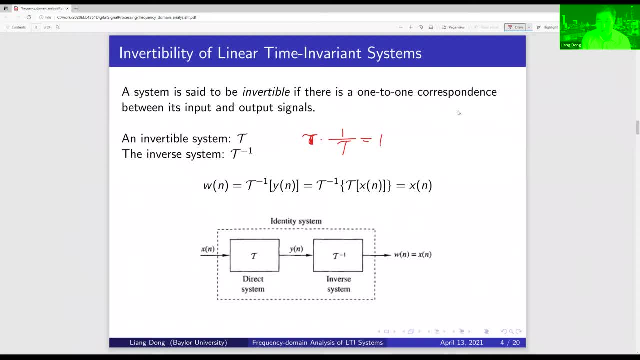 That should be one, one across all frequency. That is a constant. one is not a function, It's a function of frequency, right? So it's constant across all frequency. So the signal go through my inverse system. So we have this inverse system. 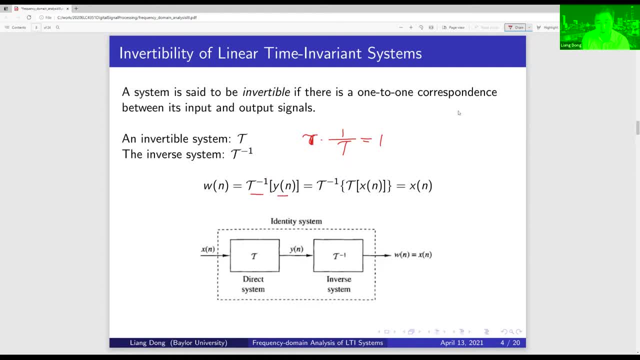 That's an operator, Operator on the output signal YN. So that is my inverse system operation on YN, YN, which is the operation on XN, And that should give me original signal XN. So the output WN should be equal to XN. 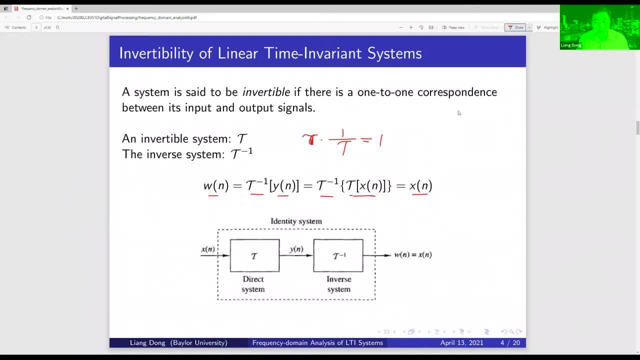 We recover the original input signal. Therefore T is indeed an inverse system. I will put in this in the block diagram. So XN, coming here, go through a direct system as T become signal. Y, Y go through an inverse system, T to the power negative one. 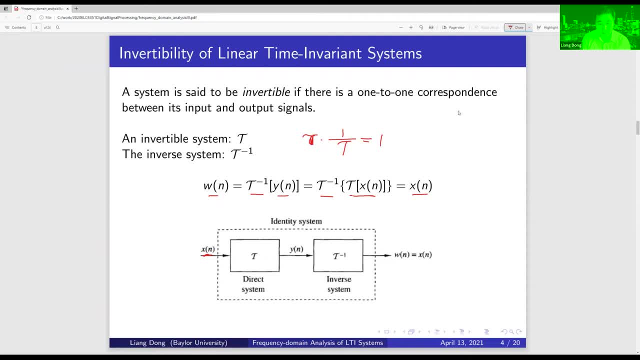 and give me the final output to WN, And we want to have WN equal to XN. Therefore, the entire thing in this started the in this box is identity system right, Everything This is. this is T negative one times T. 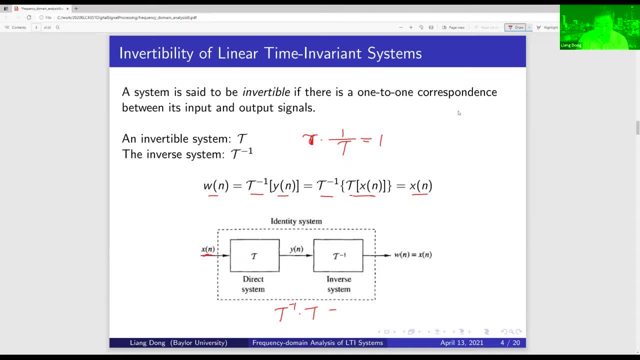 Those two operator. What should that be? Well, in the frequency domain, that is one, As we said here, that is one. What is this? in the time domain, This identity system, If I'm trying to look, entire system, we call this entire system H. 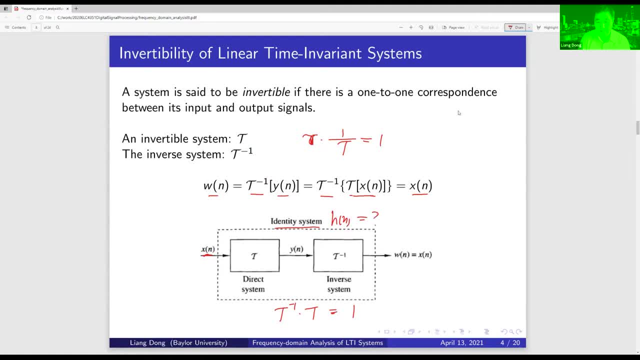 This is the entire box. What is that for an identity system? That is quite straightforward, right? When we do a inverse Fourier transform, what is inverse Fourier transform or constant, Especially one that should be equal to Delta N? Delta N- It's just a data function. 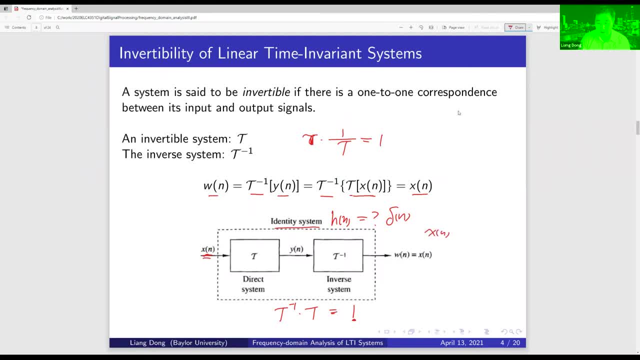 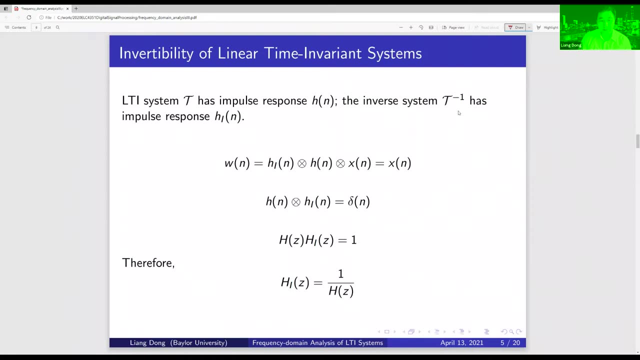 Well, indeed, XN, the input signal convolved with a Delta function. that gives me XN, So the output is still XN. Therefore, that is the identity system. The LTI system T has impulse response HN. The inverse system T to the power, negative one. 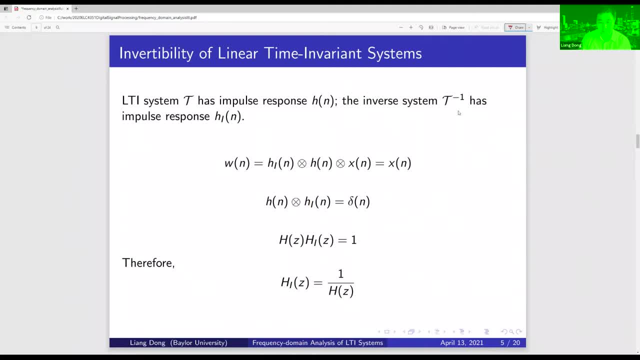 has impulse response. We call it H sub I Because WN is equal to XN, So WN is system X, signal X go through system H, go through a system H sub I. So it's, those are the two convolution. Now convolution we can associate. 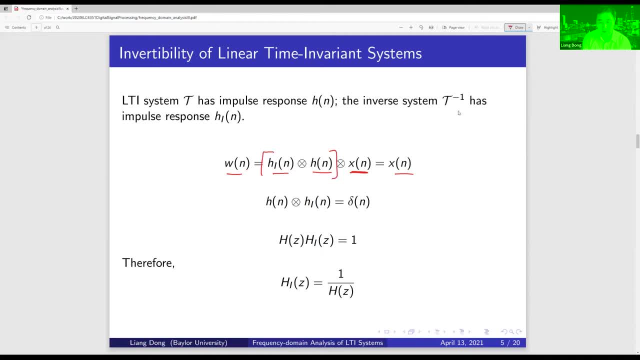 these two convolutions together. Therefore, these two give me a combined system That is the Delta function, Delta N In frequency domain. we have already seen that Capital HZ times capital H sub IZ equals to what That gives me an identity system. 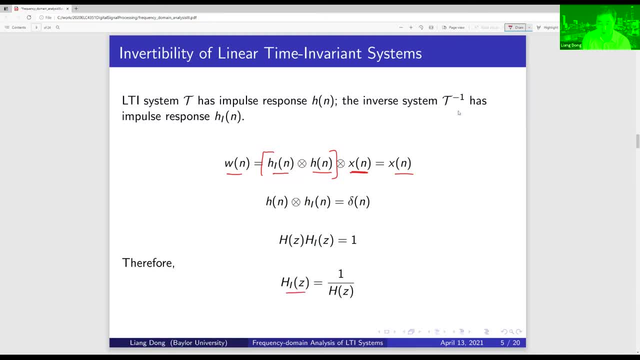 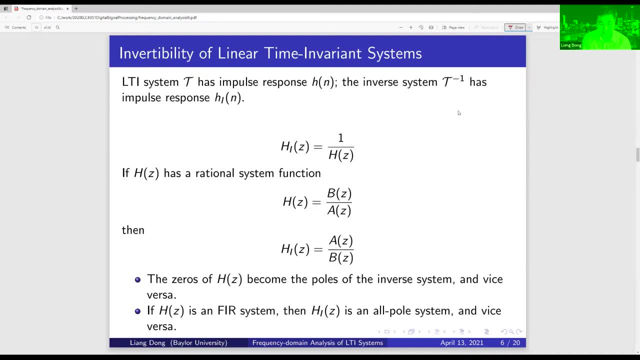 Therefore H sub I is, in the inverse, one over one over capital HZ. If HZ has a rational system function, which is the usual case for any system that is implementable, we can draw the schematic for that with A's and B's. 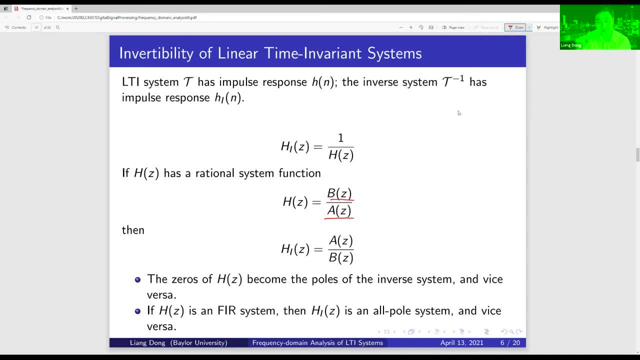 Those are the polynomials, The B's. on the numerator, that's the feed forward network, right Feed forward, we have to delay the tap And the AZ. on the denominator, that's the feedback loop from the Y and it comes with a delay. 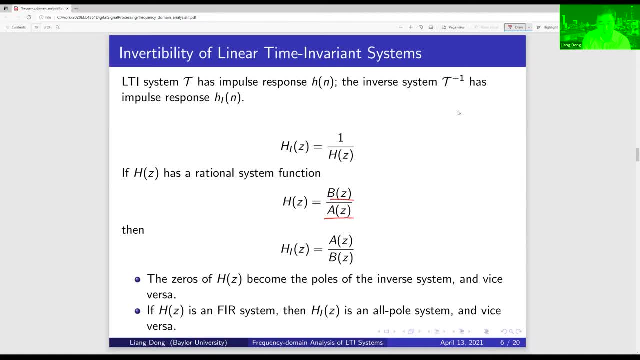 with few delays and coming back. We should know this very, we should be very familiar with these. If this is the case, a rational system function. then the inverse system can be easily expressed. We just flip the numerator denominator, So that's A over B. 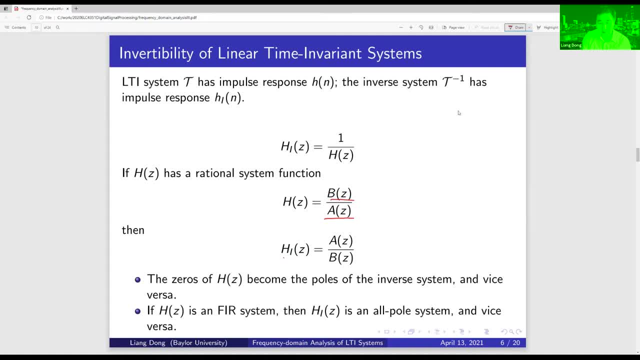 which means that the zeros of HZ become the pose of the inverse system and vice versa. right, Because I change numerator to denominator, denominator to numerator, So the zeros and the pose are exactly the exactly change their positions from the direct system to the inverse system. 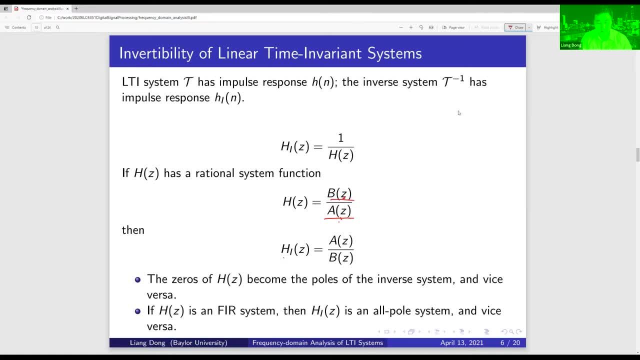 If HZ is an FIR system. if HZ is an FIR system, meaning that the system has only numerator, without any denominator, So HZ equals to BZ. this is FIR system. finite impulse response: That means I only have zeros. 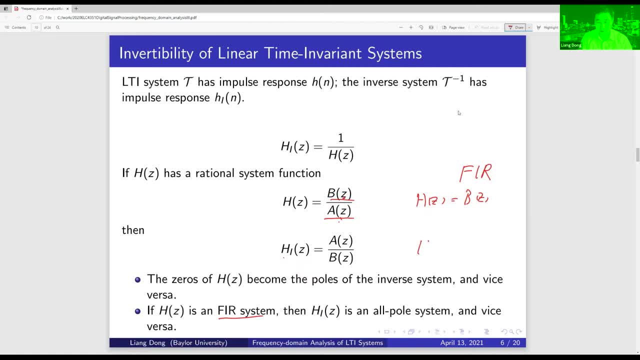 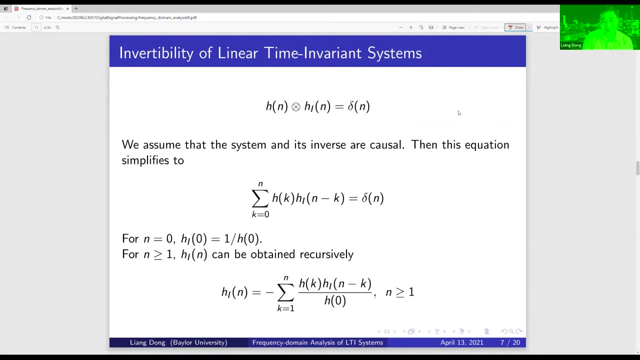 There is no pole. Then H sub IZ. that is in the form like this one: over BZ, Everything is on the denominator, There is no numeric term. So H sub IZ is an all pole system and vice versa. In a time domain we have this expression. 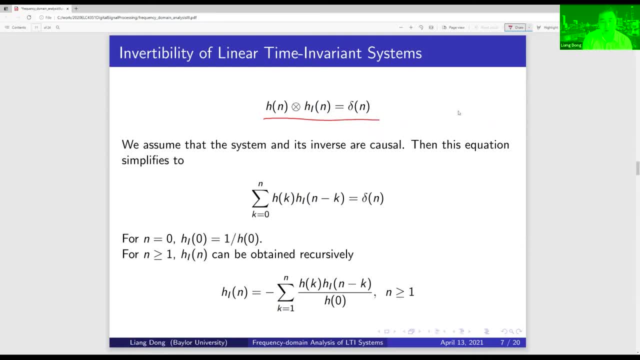 The convolution of H and H sub I is delta function. Okay, We assume the system and its inverse are causal. for any practical system it's a causal system. Causal system that the system is not defined When N is less than zero. 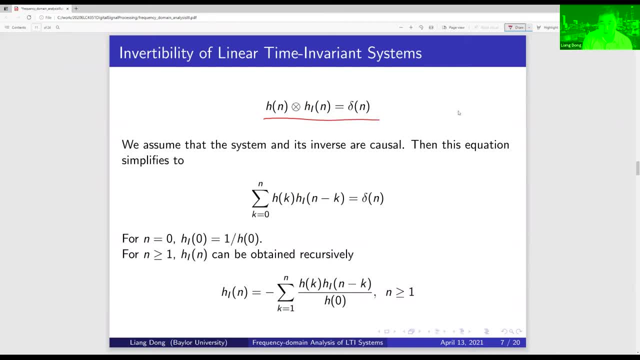 Then this question simplifies to that. This is a causal system. It's either not defined or, when time is less than zero, everything is zero. You just make everything zero. That's a causal system. So the causal system that we have, this convolution. 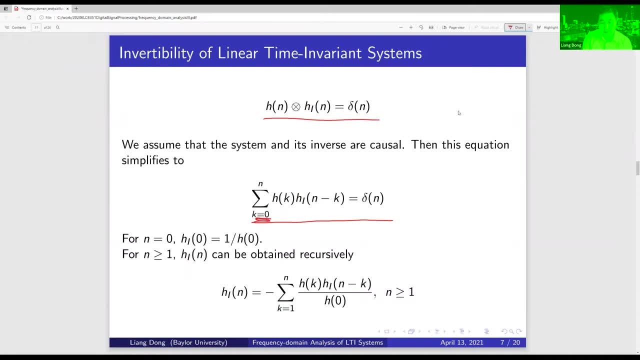 is K from zero to N. We have that. This is delta N. Okay, So how come it comes from zero all the way to N, not to infinity? Well, we are not only need to take care of one system: H. 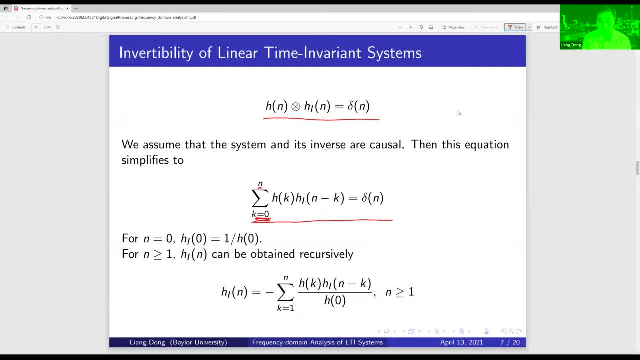 but we also need to take care of the other system. H sub I is also causal, So therefore this sum is bounded by two Ns, either zero or the current time N. So it's from zero to N, Given that we can calculate H sub I iteratively. 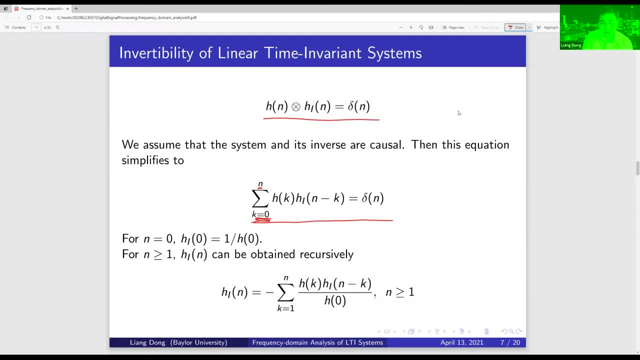 So for N equal to zero, we find out HI H sub I zero equal to one over H zero. So that is simple. because H zero, H sub I N is zero. So that's a negative K which is also zero. 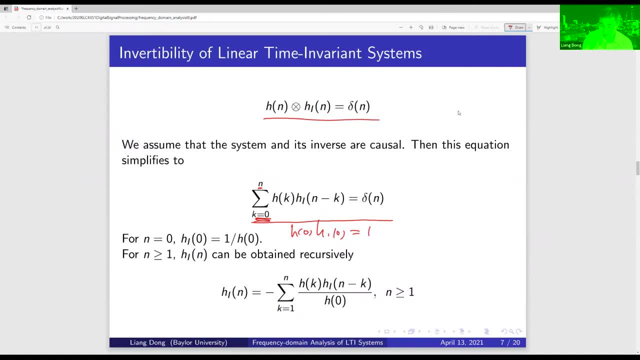 K from zero equal to one, And so we find that If N is greater than equal to one, then H sub I N can be obtained recursively using this format. I think there's a typo in the textbook. So this is correct, because from here: 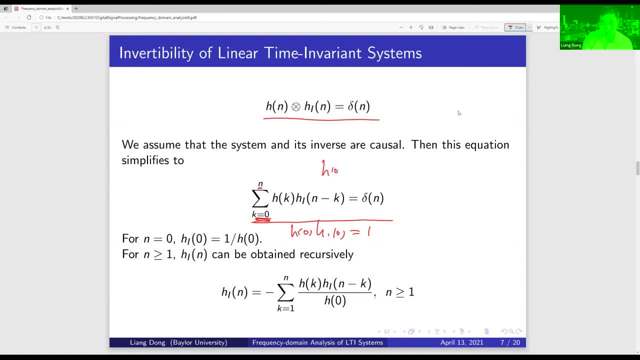 all we did is we just taking one term out of the summation, which is K equal to zero plus K from one to N, H K times H sub I. N subtract K. K equals to Delta N If N is greater than equal to one. 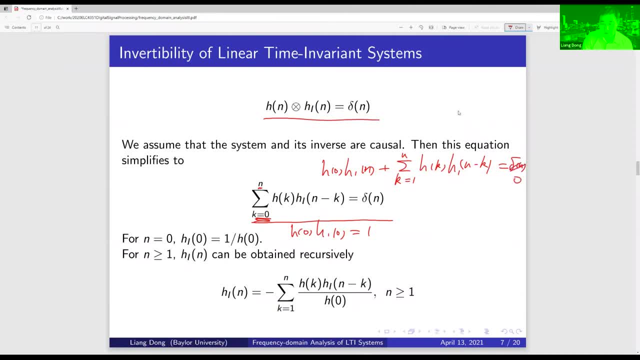 this part becomes zero. Therefore, you move this to the right of equation and we find out: HIN can be expressed in this form And that can be easily calculated for the inverter system. We have other ways to do this: to find this equalizer. 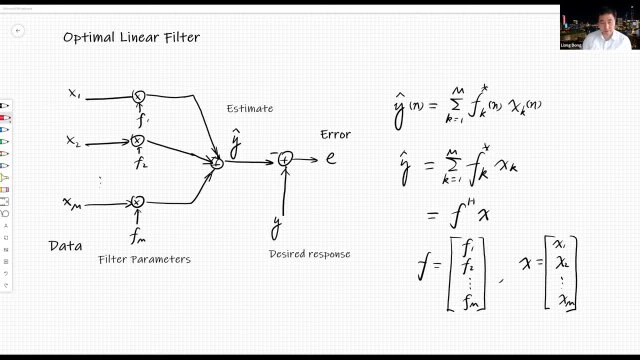 Especially, there is a method for advanced digital signal processing. It's called optimal linear filter. Let me just start it. We were going to get back this later, at a later time, to see how to solve for an optimal linear filter. So the optimal linear filter is that I have a data. 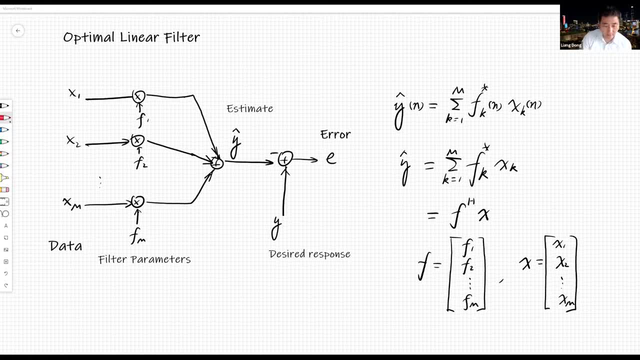 that's the input data, X1 to XN. Then I have a go through a finite input response filter, This FIR filter, with parameters F1, F2, all the way to FN. we have the output, which I call is y hat. 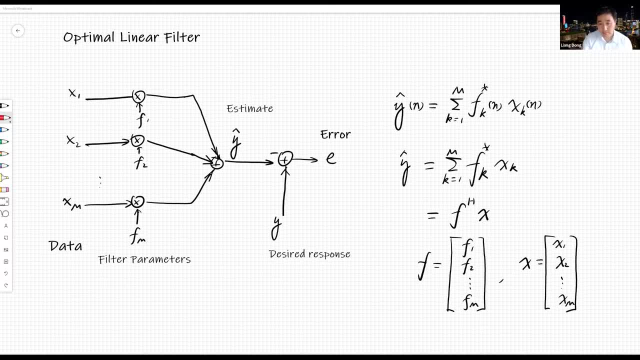 This is output of this filtering. So in the time domain, if we look at this equation, this equation here, this is a convolution. this is a convolution of a H, of a X with F and we got the output of Y. Now our job is to find those coefficients, f's and such that we have a very nice filter. 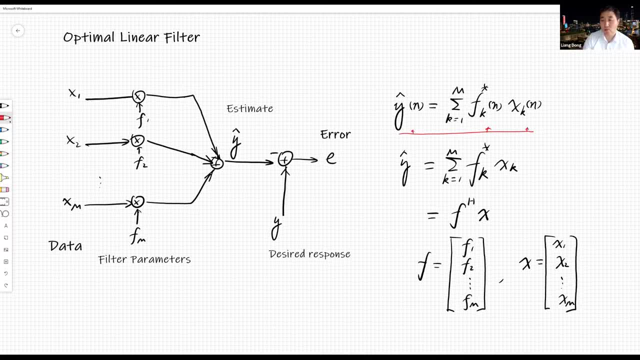 for all the x, I can estimate a y. we get a y for our purpose and that can be extended very easily to an equalizer for an equalizer for the system inverter. So we will see that detail later, but right now we just get a concept what we are trying. 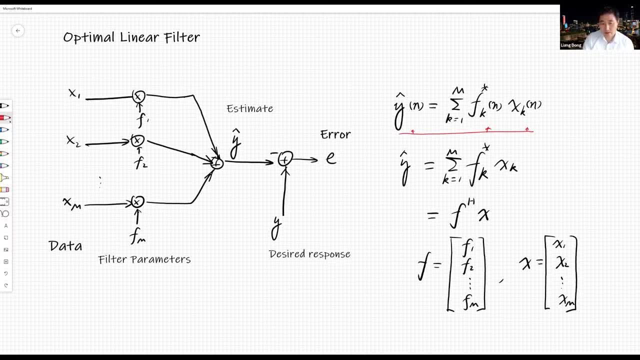 to do, And this y hat will compare with a true y. that's a desired response. I want to make sure this equation will be equal to the true one. Therefore, there is an error. The error is between the desired response and the response from the filter. 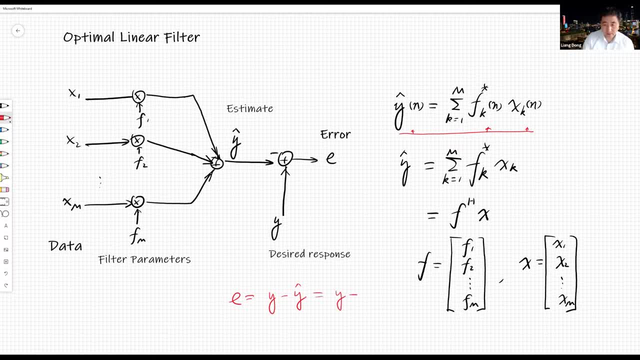 So that is y subtract f times x. f is the coefficient of my filter, x is the, the, the, the A Cyclerbing. Now what we want to do is minimize the error, but the error can be a positive, and a negative will give us a bad effect. so i want to minimize absolute value of the square, and then i may need: 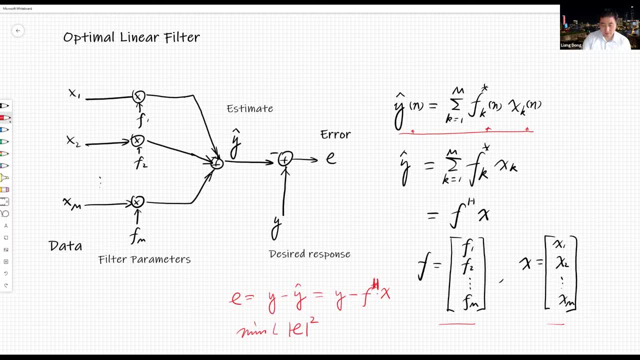 to have a lot of input signal. so i want to estimate, i want to minimize the expected value of this e square, which is in the complex format that expected e conjugate times e. we want to minimize that. minimize that with respect to variables f's. with respect to variable f's. 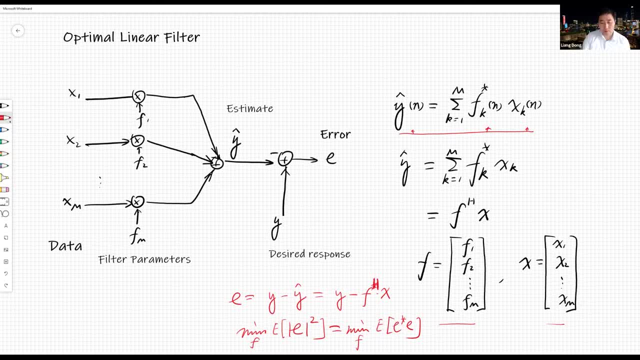 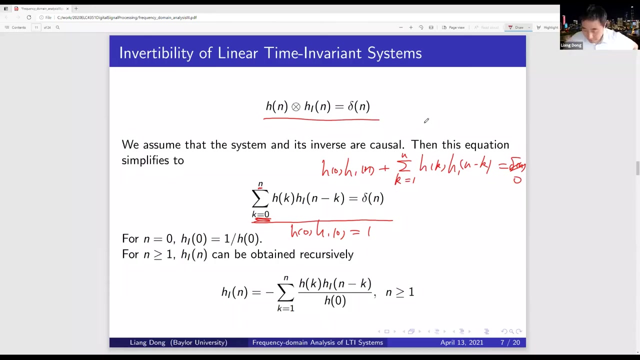 this is called the minimum mean square error optim optimizer or the linear filter, and that can work very well to find the best equalizer, to find the best invert system, and we will see that later on. so let me get back to our chapter. okay, so i'll just leave it there. give us some a good feeling, a step. 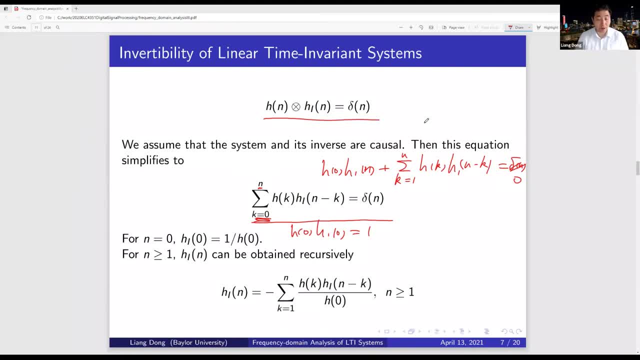 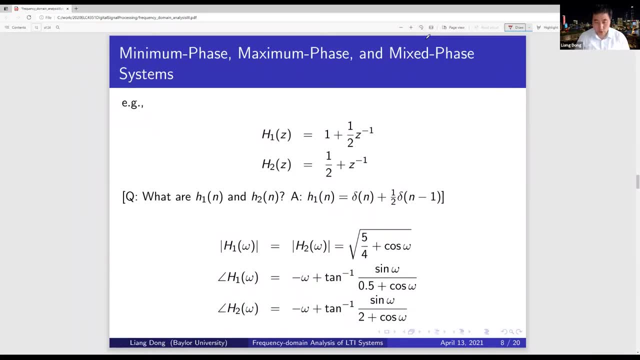 beginning step. then we will revisit that idea for optimal linear filter later. now we are getting to a concept which is called minimum phase, maximum phase and then mix, the phase of a system. phase is another, is another part of the filter. we are not only looking at amplitude but we also want to look in phase. 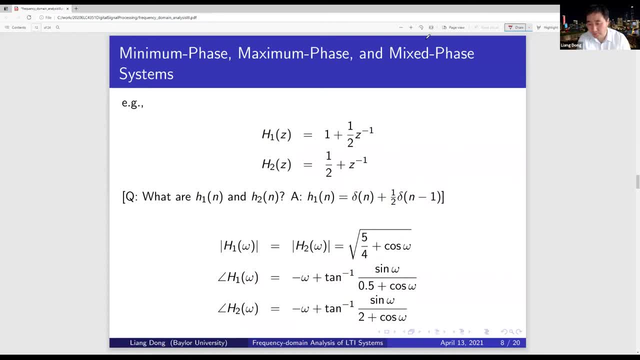 for amplitude. we know we can have a low pass filter, high pass filter, band pass filter, and that is all looking at absolute value of edge, the amplitude. what do you want? what kind of signal of high frequency or low frequency you want to emphasize? but there is also a hidden element, which is the face. we don't really see that. 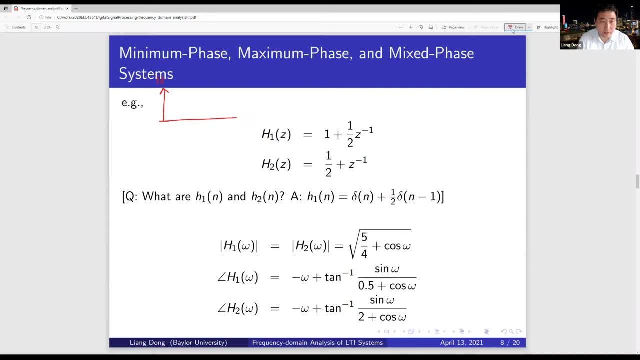 When I produce image, we have each absolute value. So for low pass filter it goes like this: from zero to pi. But there is also another element we are not looking carefully, which is the phase, which is angle of h omega. 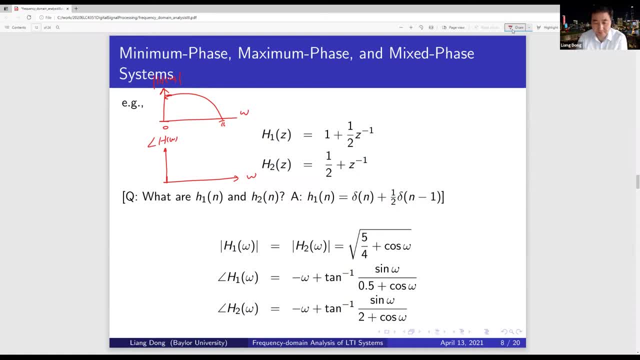 We said something about the face of a filter. When we mentioned that, we mentioned something about a linear face. right, We want to have a linear phase system. We also mentioned the group delay. Group delay is the derivative of the phase, So in this case, if it's linear, then the group delay is a constant. 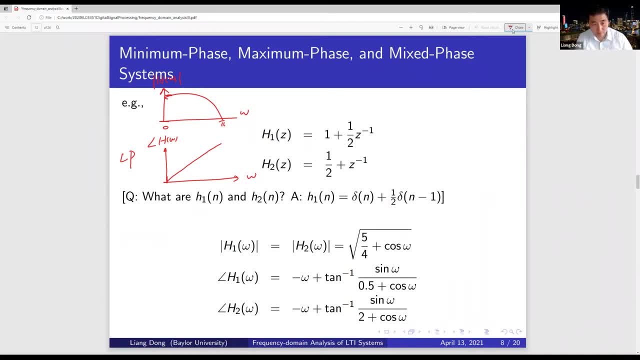 So now we look into this phase issues to see how we can relate this to a system and what kind of effect that it will give us. I have two systems here. Two system is h1. And h2. As given on this page, those two example- h1 is in the z domain, one plus half times z to the power negative one. 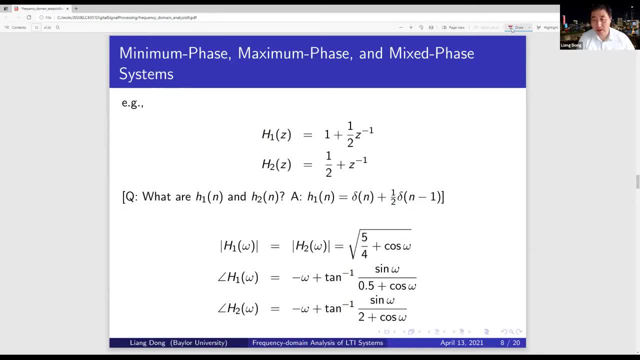 h2 in the z domain is half plus z to the power negative one. So what is the in time domain h1n and h2n In time domain? this is delta n plus half times delta n minus one. This is half plus delta n plus delta n minus one. 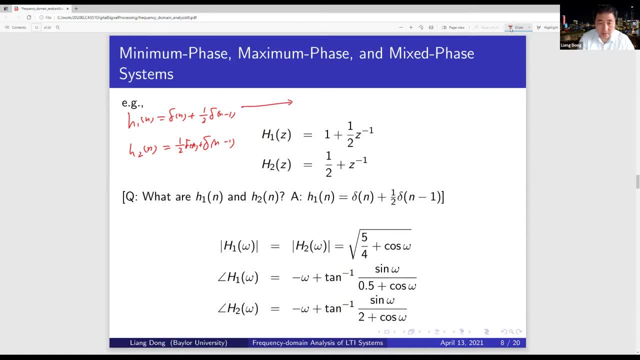 So in the picture we see that the first h1, it looks like in time domain, that is a delta here, And then I have a half here. This is zero, This is at one, This is at one For h2 time domain. we have a half here. 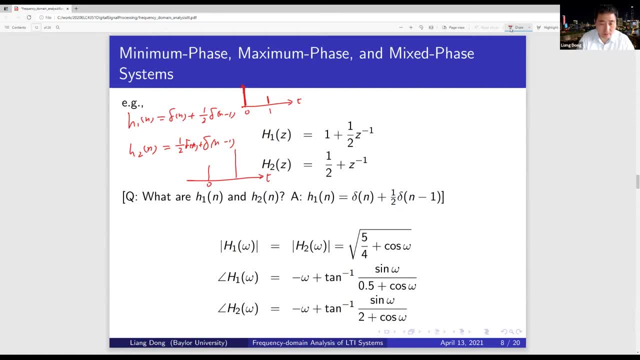 This is a zero, Then I have a one here at time. one: This is a half. This is a one. This is a one. This is a half. All right, It's a. it's a delay system, And so we have a delayed tap. finite impulse response. 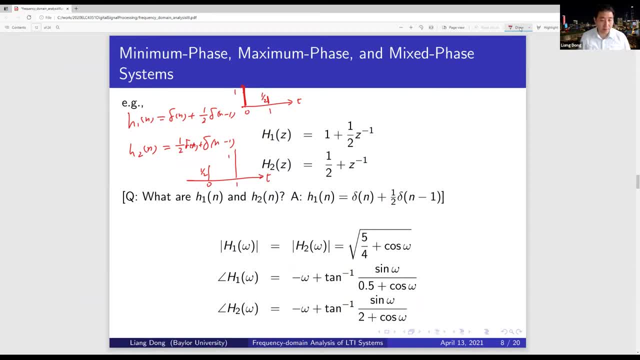 All right. So in the frequency domain, we will see that this delay element, this delay element will give us frequency selectivity. So capital H, capital H2, we will have an angle. That angle is not zero. We also want to find, we also notice here. 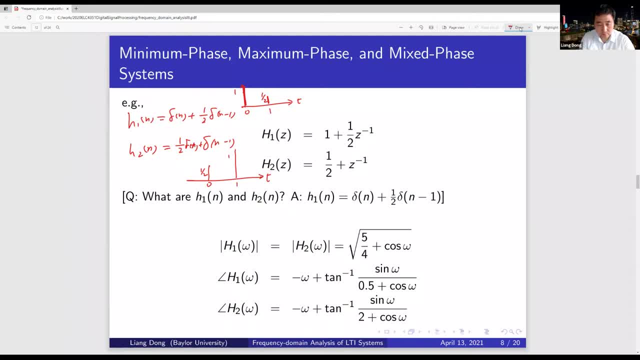 Now compare these two systems. Which system or which filter is a better filter? It's hard to say, But just by looking at those two delta functions we see that. well, maybe H1 is better, Because I have a delay path here is smaller. 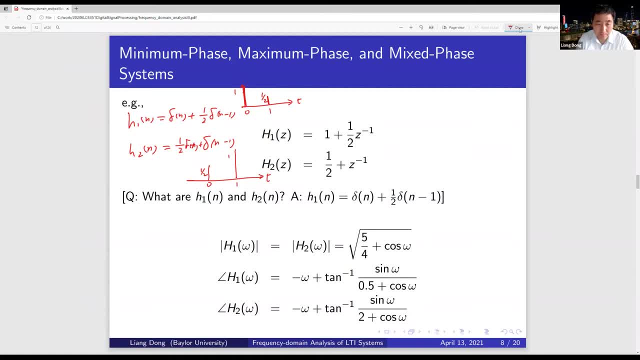 I want to concentrate all the energy at the at this non-delayed path, Or we concentrate the energy of the filter as much as close to zero. Therefore I don't have a heavy delayed tail right. So you have the input X and given Y, Y and output. 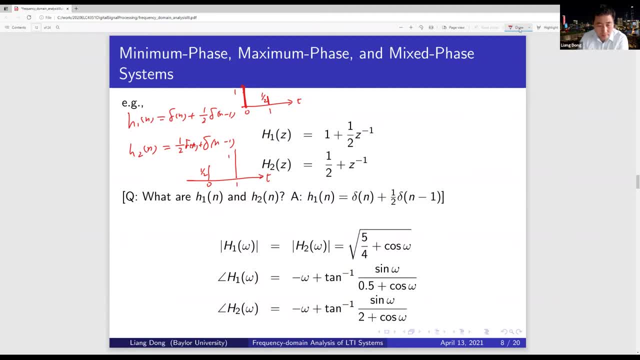 You don't have too much of the delay effect. Now compare with the second one. the regular incoming signal through this filter, Xn, becomes half of Xn, But you have a delayed term. This delay term is relatively large. You have a large delayed or it's a large tail there. tail effect. 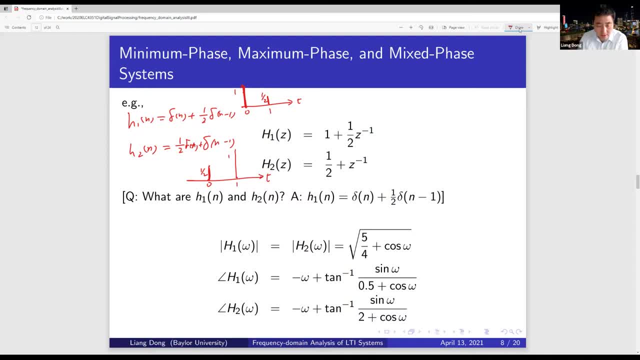 And then it seems that if I have the energy of the system kind of dispersed into a large time, a large delay, maybe it will give me a more, a worse effect on my input signal Xn. So we keep that in mind. Let's continue to see, look at, to examine H1 and H2.. 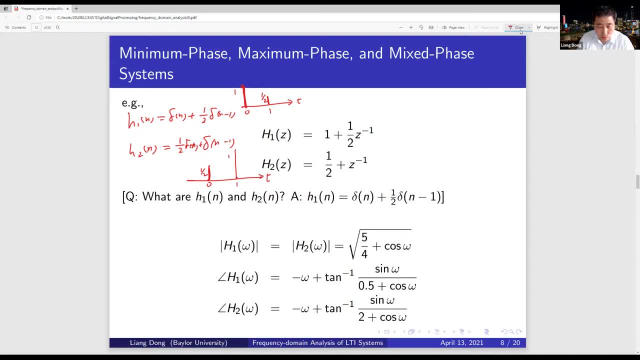 All right. so what is the amplitude of the frequency domain signal like this and this Absolute value of H1, absolute value of H2.. To calculate that, let me just work on one part. Let's see H1.. Omega, H1, omega is here, is one plus half. 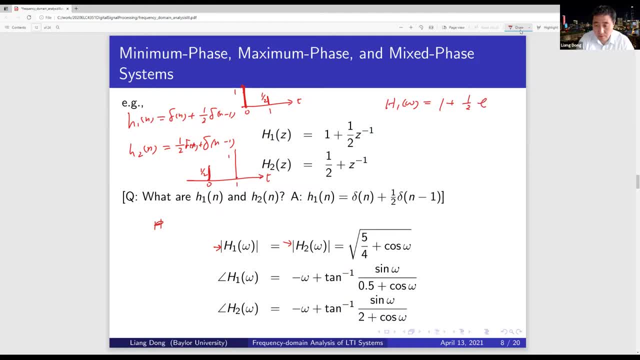 And then we have: here is e to the power, negative j omega, And this will give us one plus half a cosine omega subtract j sine omega Here, And so the real part is this. And then we have the imaginary part here: j omega. 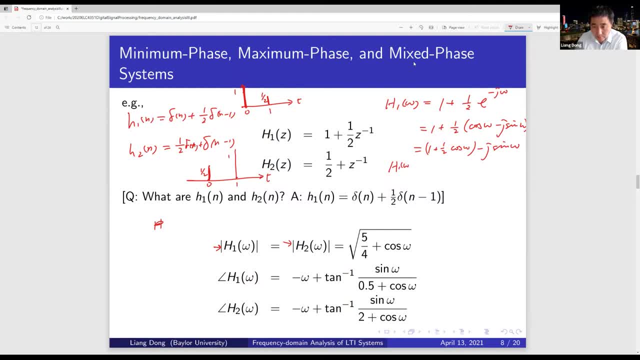 To find absolute value of H, That is equal to one plus half a cosine omega square Plus sine omega square, And then take the square root So that we have- let me just do a few steps here. That's one plus cosine omega plus one over four. 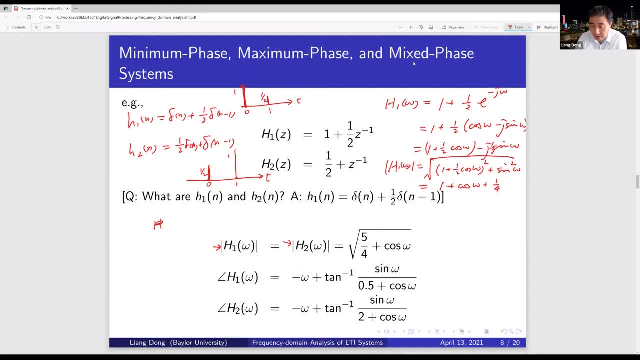 Excuse me, Excuse me, I have a half here, I have a half here. So this is one over four here. So one over four cosine square, Cosine omega square, And plus one over four Sine omega square. 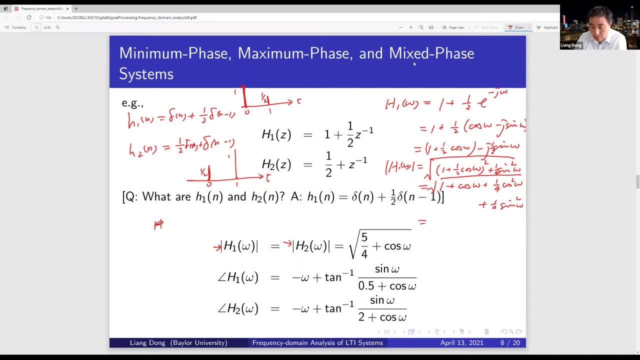 And then take a square root here, That will be square root of One plus one over four Plus cosine omega. All right, So that's what we have here. The amplitude is equal to that Now if you calculate absolute value of H2.. 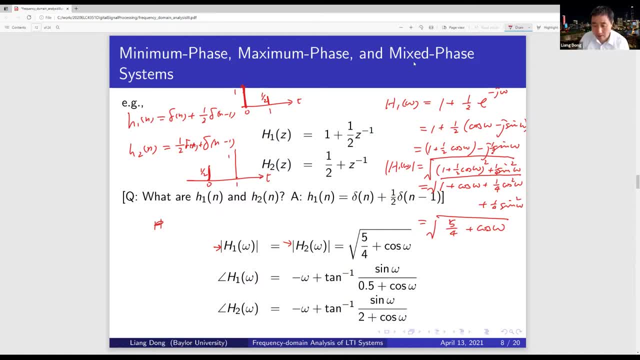 You get the same result. It's five over four plus cosine omega Square root. From the amplitude part, I cannot see any difference between these two filters, However, From the face Element, If we looking at angle of H1 and H2.. 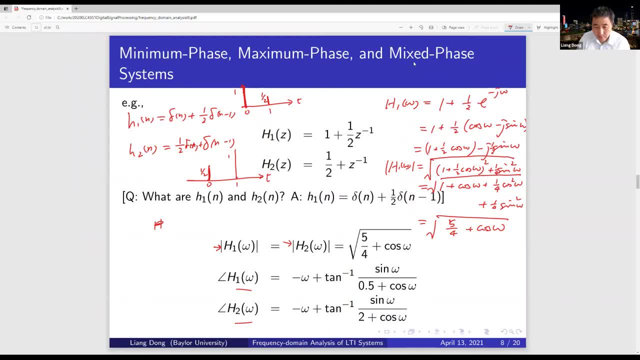 They are different. Now, how to look at those two face. Well, the face is In this case is: You can either working directly on this real part, Imaginary part, Or you can do it All. right, Let me go back. 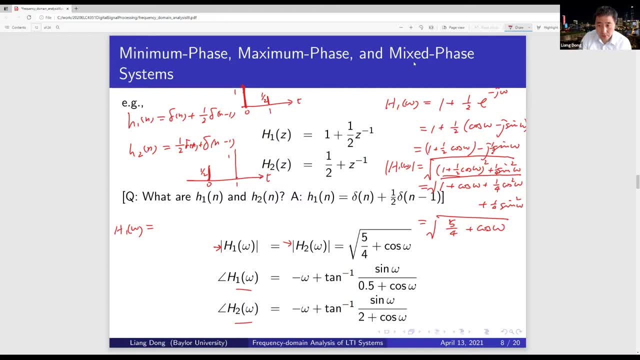 And I'll show you. So if I do this, All I can do is H1.. Omega Equals to Eat to the power J or make up Times. one Times Eat to the poetry or maker, Plus One over. 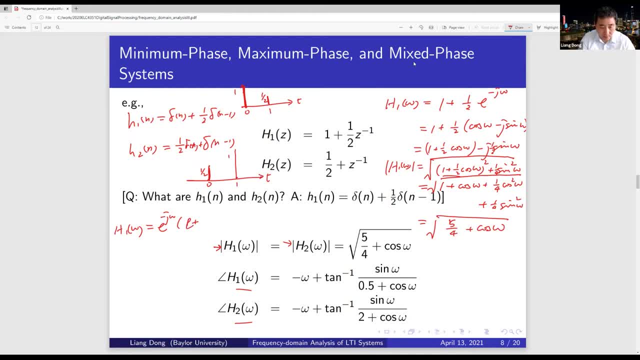 Two. Okay, Like this, I'm simply Moving Into the power. Next Is One Over Three. Okay, I think there's actually an e to the power, negative j, omega to the front out of this parenthesis. so we calculate the angle. 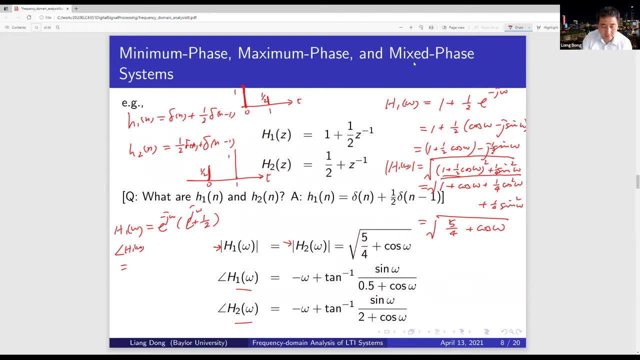 of h1. so the angle is the first, this part, the angle is negative omega plus the angle of e to the power j omega. and i have right now the second part here is: is a cosine omega plus sine, j sine, omega plus half and go of that so that is equal to negative omega. 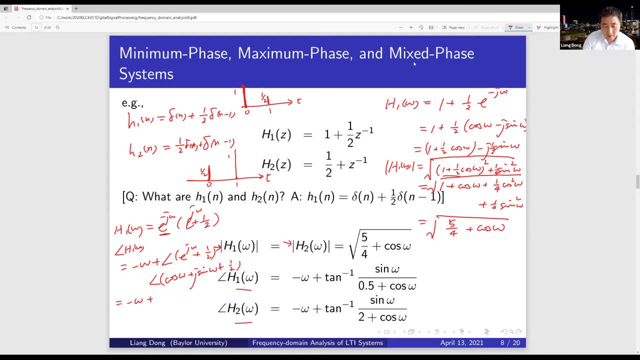 plus and to find this phase, well, it's a, it's arctangent écingent of the inhibitor of energy, imaginary part, which is sine omega over the real part. here is 1 over 2 plus cosine omega. okay, therefore, i got this result. this is result is here, exactly here. 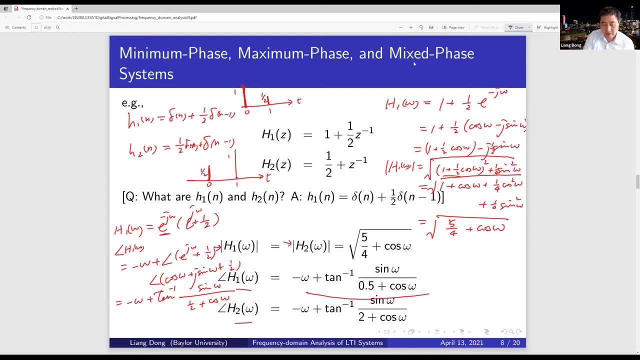 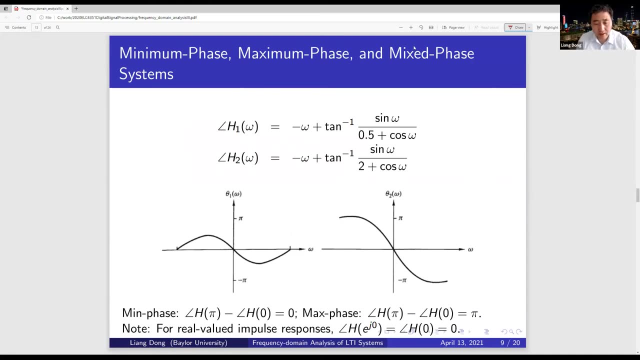 if we calculate the angle of h2, we find out it's different. it's different. we got some part here is different. let me rewrite those two face values, those two face values, if i plot on the image. this image is with respect to frequency outcome. the y-axis is the face, the angle of h1 and angle of. 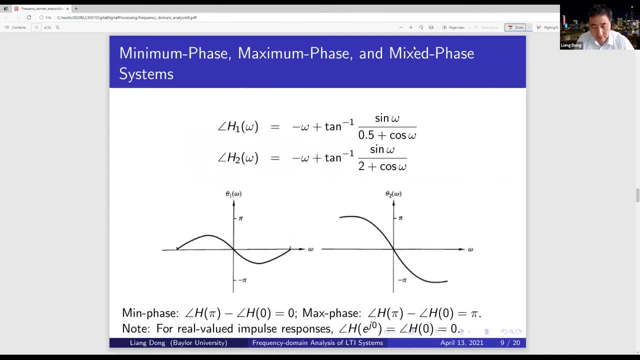 h2. we find out those two are different, different curve, and those curves are not linear. they are have this curvature effect. it's not linear. The first one is look like this: It goes through origin and it will end at zero when omega equal to pi. 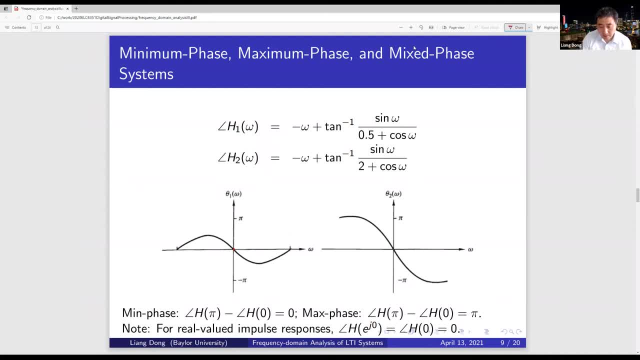 The second one goes from origin, but it will end at negative pi when omega equal to pi. We call the first part, we call that a minimum phase system. A minimum phase system is that we only look at those two extreme, end at frequency pi versus frequency zero. 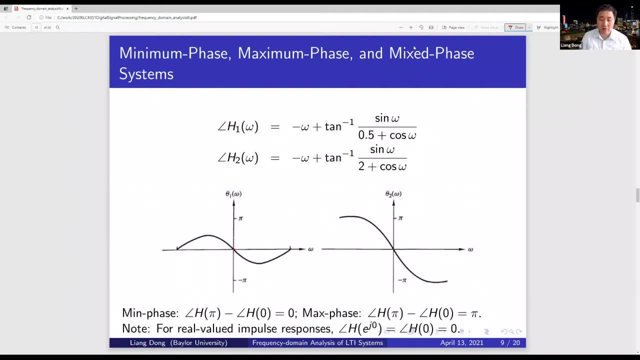 If the angle at frequency pi subtract the angle frequency at one, at the angle at frequency one equal to zero, we call that a minimum phase system. If the angle of the system at pi subtract the angle of system at frequency zero equal to pi, we call that a maximum phase system. 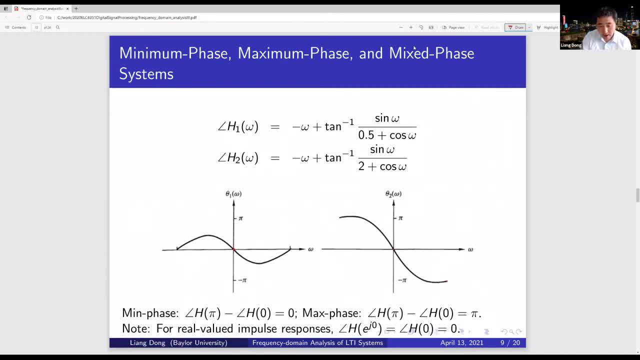 OK, OK, And for the real value of impulse response: if impulse response HN has all these finite impulse response, for example that I have, all these H1, H2, H3 are real numbers, Then we know the HN is a complex symmetry. 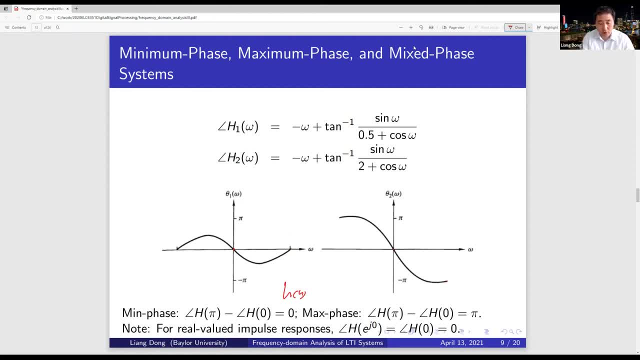 It's a complex symmetry. Therefore it has to go through the origin. The phase has to go through the origin. Therefore, the angle of H when omega equal to zero, That is, angle of H0 equal to zero, That has to go through the origin. 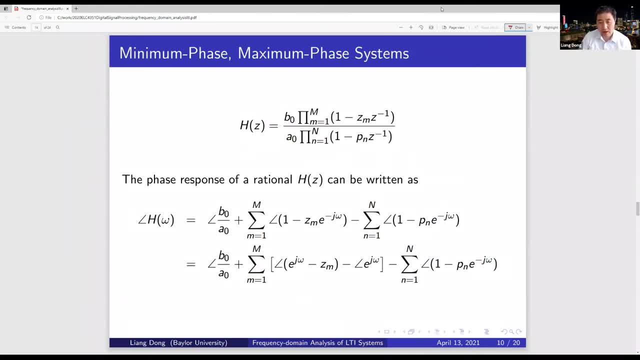 To look at the effect of the phase. let's look at how to find this phase angle, And we are using a picture to find a phase angle in this general format. Then we look back into our specific examples of H1, H2 to see why we call that minimum phase and a maximum phase. 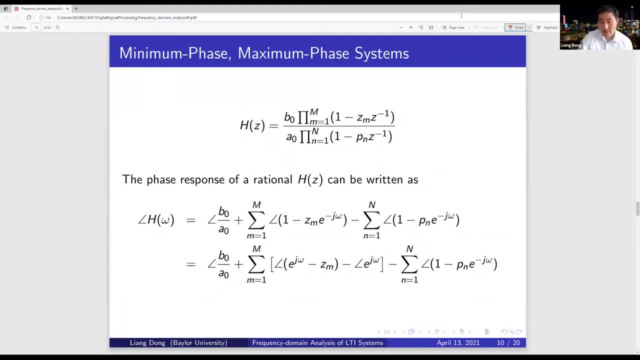 So in general a linear time invariant system can be expressed in this rational format. So HZ we have here as a polynomial on the numerator and a polynomial on the denominator. So we got the zeros and the poles. The phase response of a rational HZ can be written in the following: 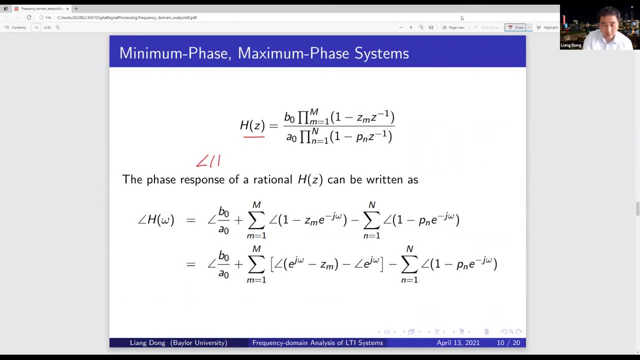 So the phase is the angle of H, omega. We are looking at a phase first to this term. So we multiply by this term of the entire thing of these two products. multiplied by this, This is a constant. So if I'm calculating the phase, so I'm putting the phase of this constant first. 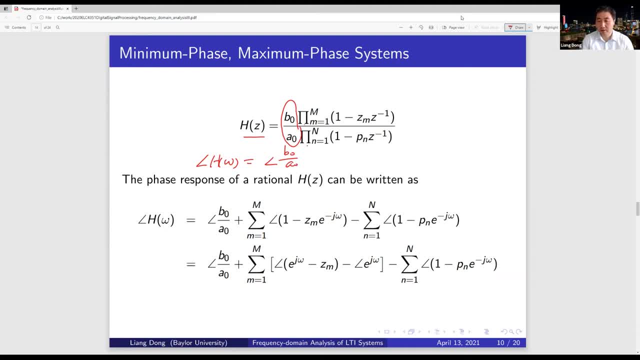 It's not a function of omega, So the phase itself is a constant. Then, plus the entire phase of this rational format which is a product of all these zero terms and a product of this pole terms. OK, similarly we can. we can separate these. 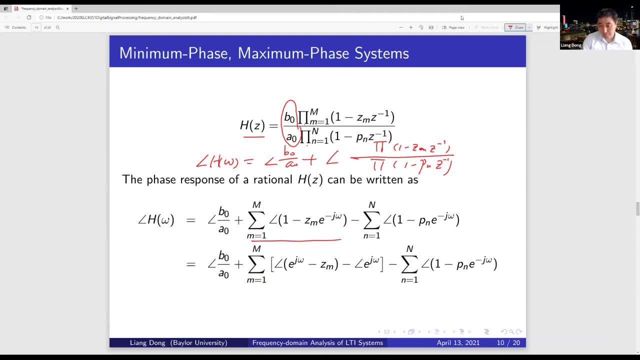 This is an angle of the numerator, the zero terms subtract because it's division, So subtract this angle, This angle of this denominator terms, And then it's a product for the angle, It becomes a summation, So summation, And then we calculate the angle of all these individual terms. 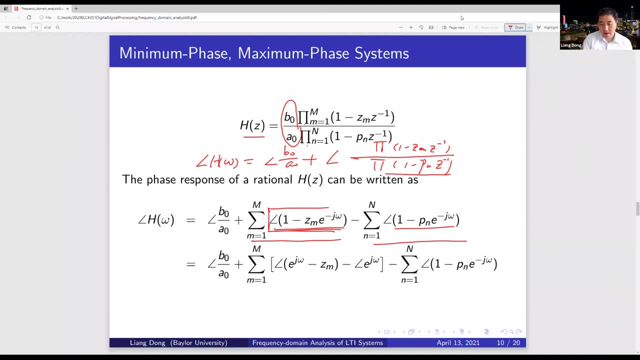 So let's just look at the first part here. So what is the angle of this? This is as we did before. Now, one subtract, C sub m times e to the power, negative j omega. That is equal to E to the power, j omega. 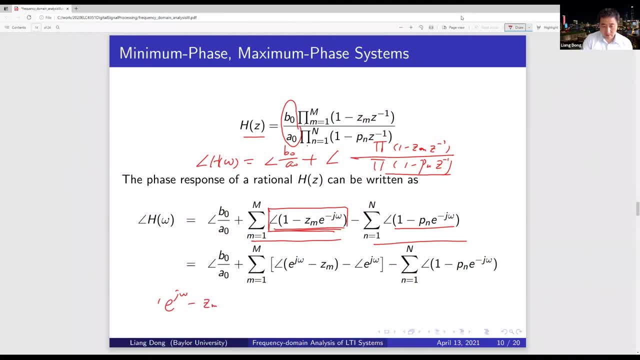 Subtract C, sub m Times e to the power, negative j, omega. This is the same as in the box. Now, if I put in an angle here, So that will be the, That will be this term, So that will be the angle. 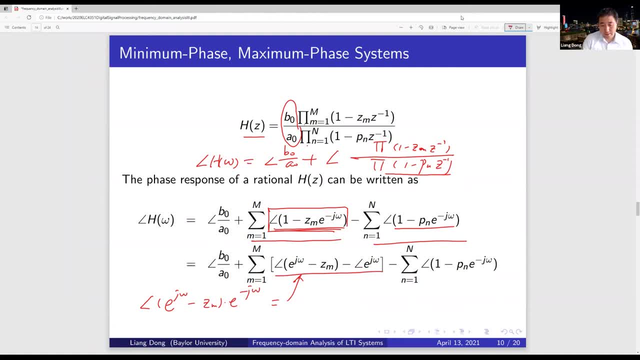 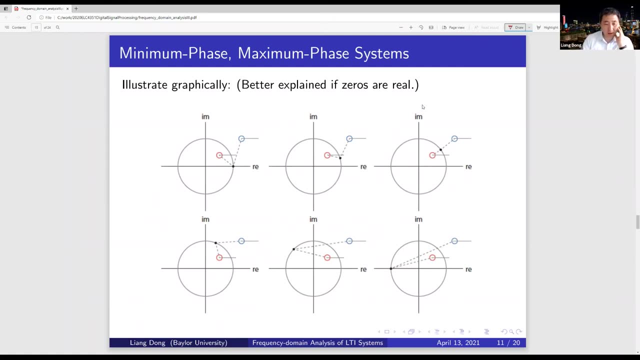 Of e to the power j omega. subtract z m. Subtract The angle of e to the power j omega, Of e to the power j omega. And what is? what is this, If I'm looking that into, On the on the Z plane, a complex plane? 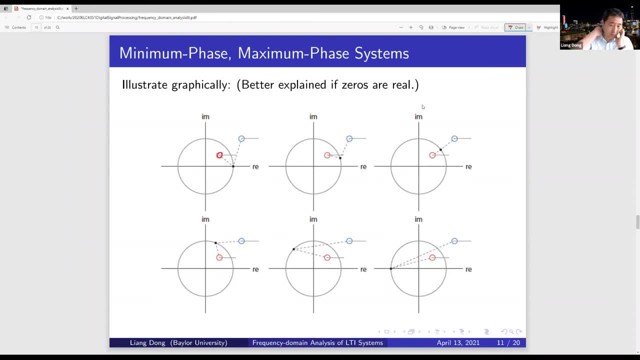 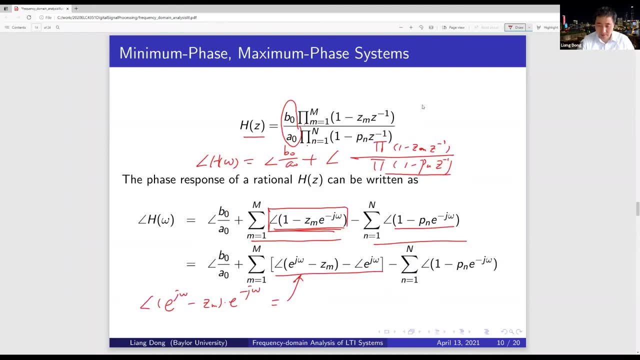 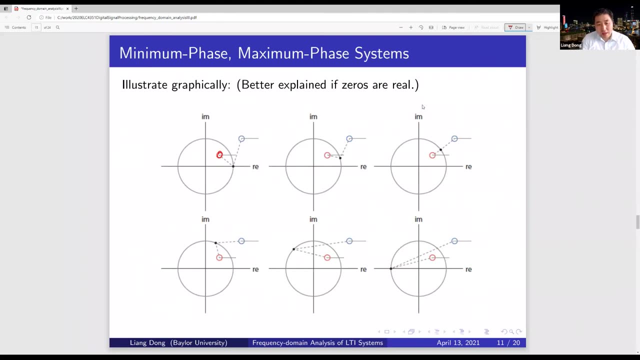 Now the, the red one, These are the, These are the zeros, The blue dots are the posts. So we are looking at the dose. This one is- Let me using the previous, Let me putting No space here. So the the point here. 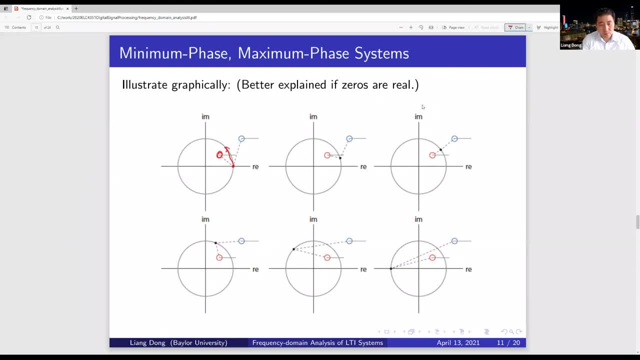 It go on the unit circle. This point Is e to the power j omega. The point here Is ZM, Right. So what is This angle? This angle is: You have C, E to the power j omega, Subtract ZM. 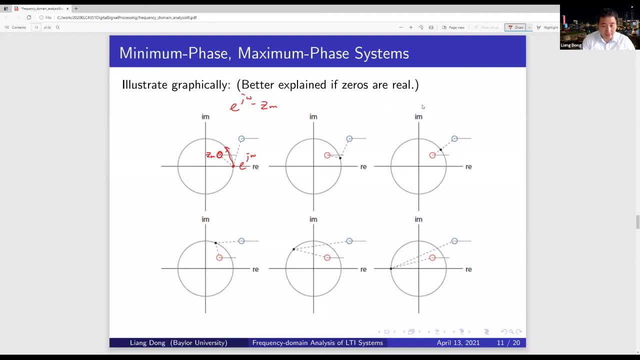 So we are looking at a vector That is on the complex me, That is a vector A pointing To Z, To the power, j, omega, That this vector Right, And then, in this case, That is this vector, And then we subtract another one. 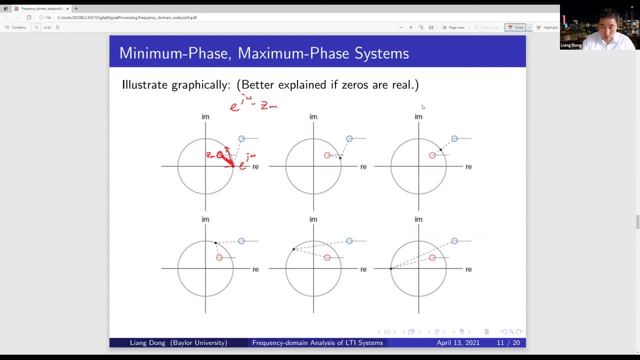 Which is Just E to the power j omega. The other one is this point, And in this case the angle is, Is zero. This angle Is, is is here. Let me Exaggerate here. So this is: 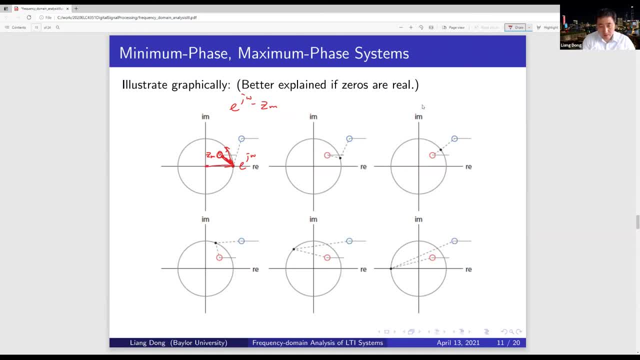 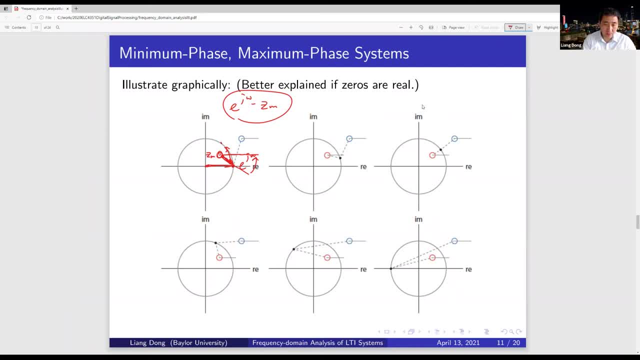 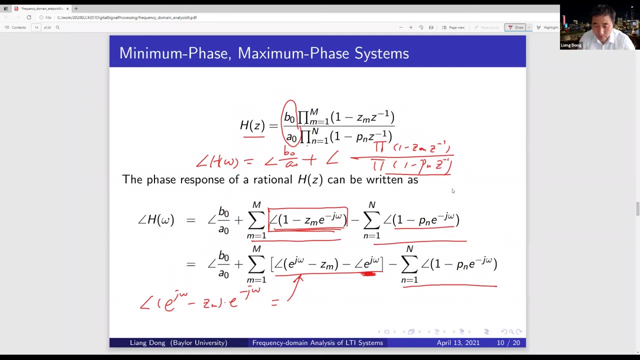 Same as If you go on This unit circle, You will also have this effect. Okay, So now To calculate The previous one, The previous one, We have another effect, which is coming from here, Of a pole. So if you combine these two, remember that's in. 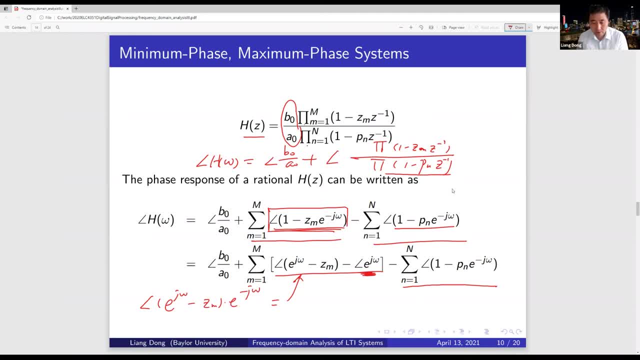 In theory we have the same amount of zeros in the pose. If you don't show that point, the point simply deform onto the origin, that is, the middle of your C plane. but we have those two parts, So if I have this part I will have another part here. Therefore, the pose is similarly. 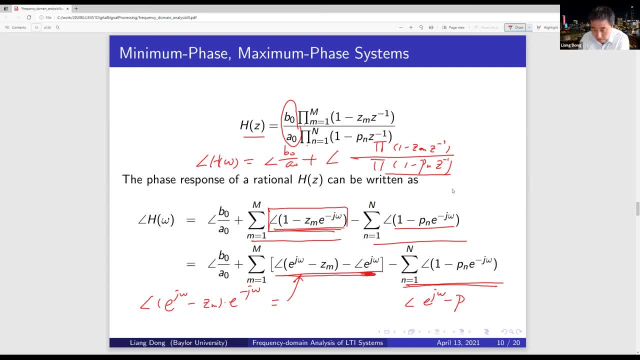 I have e to the power, j, omega subtract, p, n subtract, an angle of e, j, this part right. So if I compare this, let me use another. if I compare this one with this one subtract, so that will be cancelled out. So what's left is only the angle between your current point to 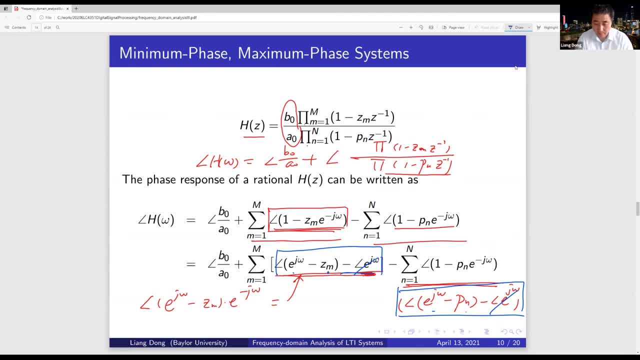 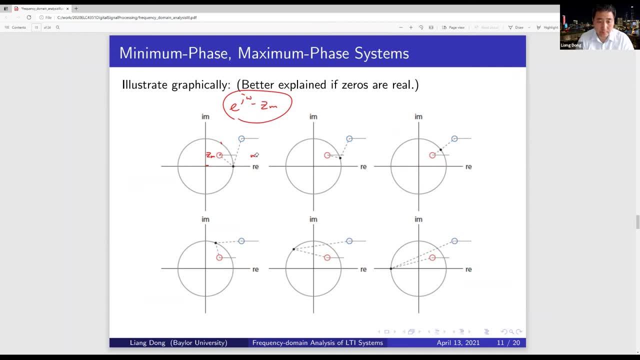 the zero and the angle of the current point to the pole, which is here. this is the. here is the angle that's between we are finding the angle of this vector, also the angle here That's how we see the distance of that And we are using that to find this, the face. 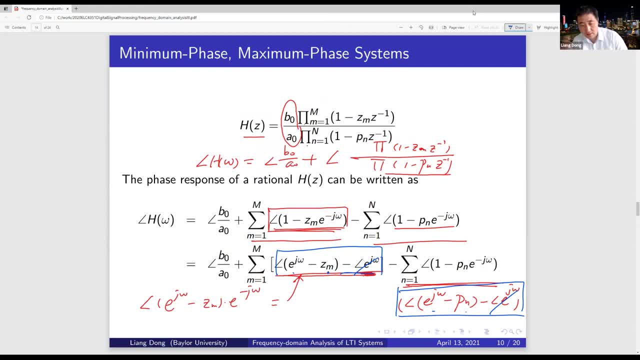 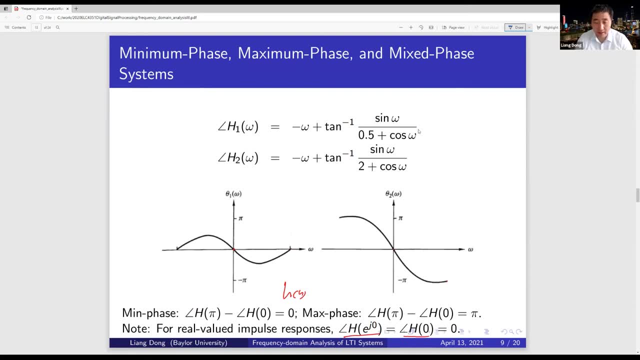 So, in general, that's how we see how to visualize this angle. Now let's look back to our case. Our example is simpler. Now let's see if I can, using this to explain the minimum face, maximum face issue. So in this case, 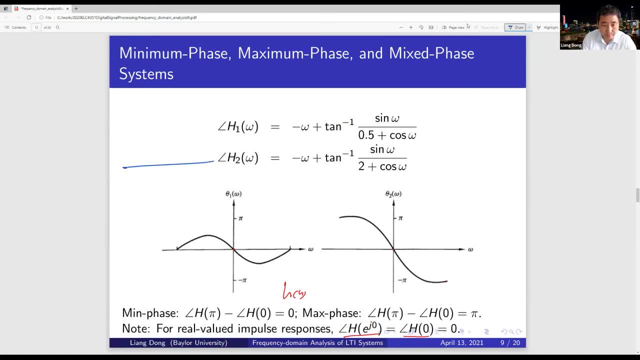 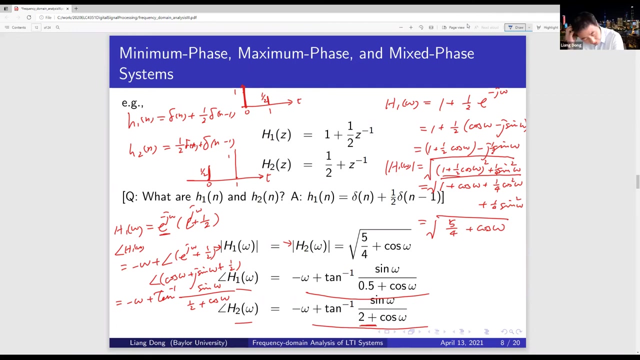 I have the unit circle here. I have two posts for my system. Let's take an example of h1, z. What are those two posts? Excuse me, the two zeros? It's an FIR system. The posts are deformed onto the origin. We don't have denominator, but we have FIR system. We have zeros. 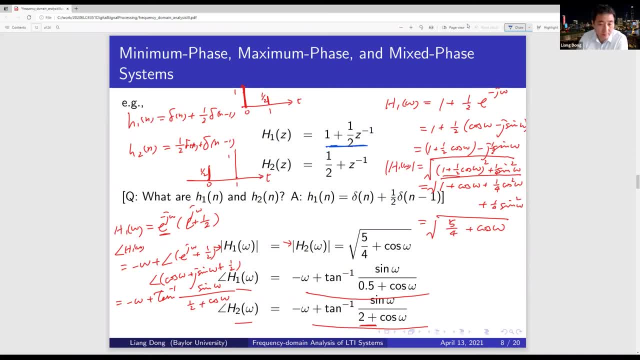 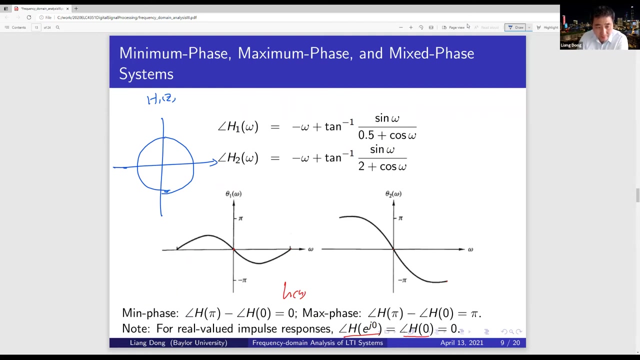 For this system, h1, I have a zero at one over two, negative one over two. For h2, I have a zero at two. Right, this is these are the first order. these are the system, the FIR system. I only have one delay. So for h1, z, I have a zero here at negative, one over two. 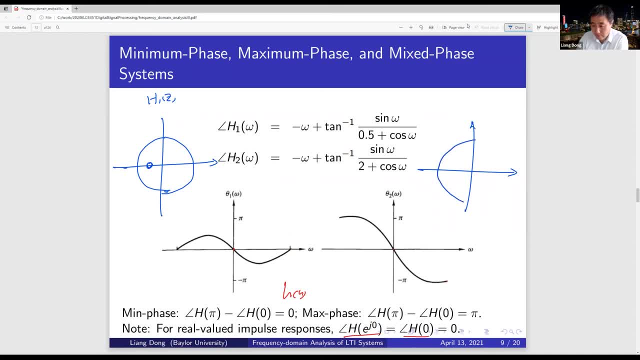 For for h2, z. I have a zero here at negative two. This is the z plane. Now, if I have a signal and travel along on this unit circle, so that will give me a frequency domain signal which is h omega. with this, this is my omega value. 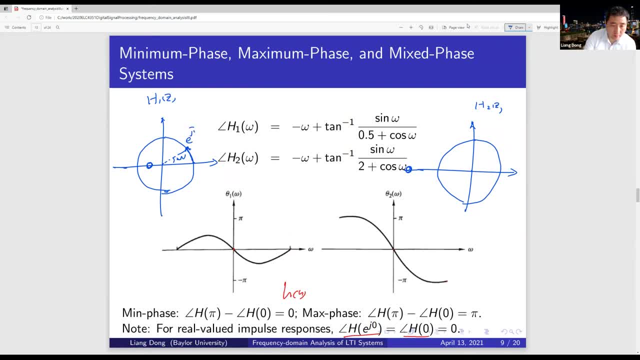 This point on here on the unit circle is e to the power, j omega. Focus on the angle of h1.. We have here this: h1 is equal to that. that's e to the power, j omega times e to the power. 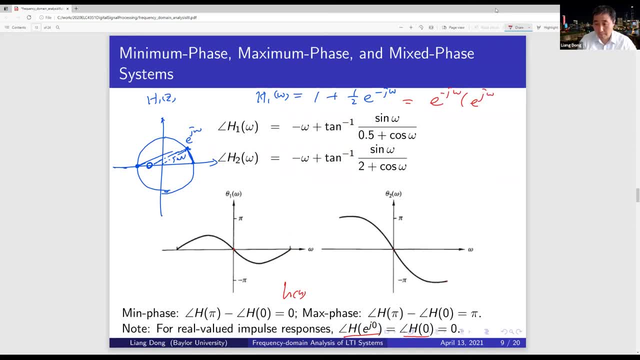 a negative omega times e to the power j omega. subtract z1, right z1 is negative one over two. so we have that, This is what we have right here, right here, right here. and therefore the angle of h1 omega is the angle which is negative omega. 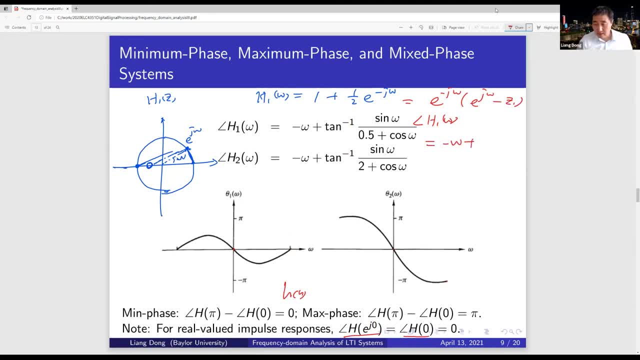 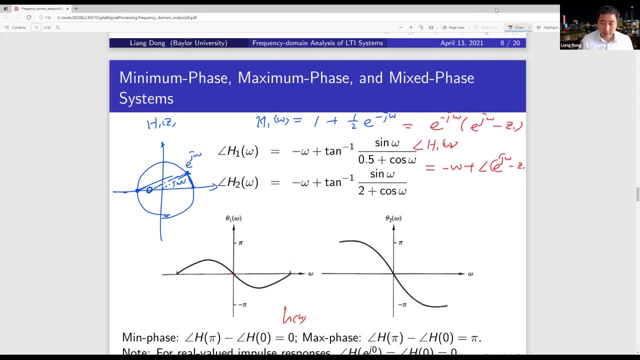 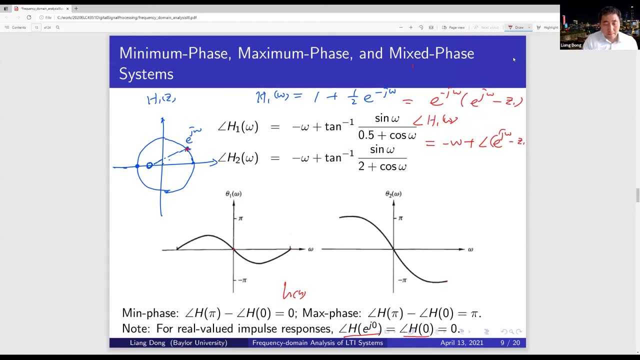 plus this angle here, which is the angle of ej, omega subtract z1. okay, so we are looking at those two parts now. if i am adding at this point, this is e to the power j, omega. the first is this: the angle of this factor itself. so the angle is here, this angle is omega. the second angle is the angle. 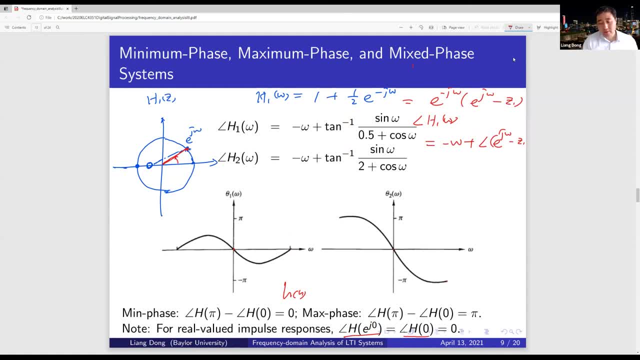 between this point, e to the power, j omega and the zero, the first zero, z1, and it's pointing to this angle here. this angle is right here, this angle is right here. that's the second part. the second part is the, the difference of two complex vectors: e to the power, j omega and then z1. therefore, it is. 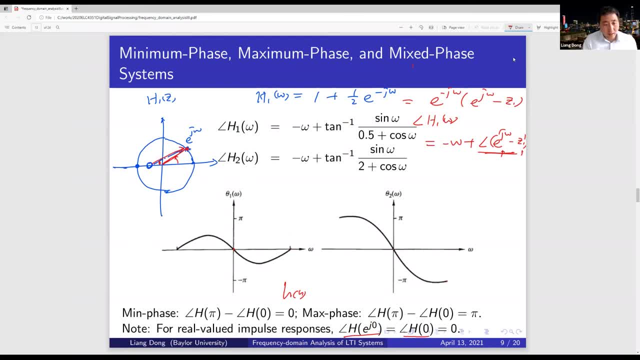 this line here. this is the line here and the angle is here. the difference between these two from geometry we know this is the angle is it is right here, right. so the angle, the first angle subtracted the second angle, that's the angle right here in here and we have a negative sign. So actually, 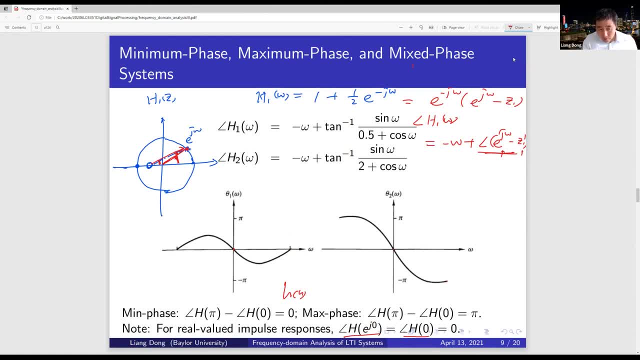 it's negative sign, the negative of this angle between this zero and the origin is right here. Okay, so with that, now let's check what will be the largest time of this angle in absolute value sense, is when I travel on this circle, when I get to somewhere here in the middle. 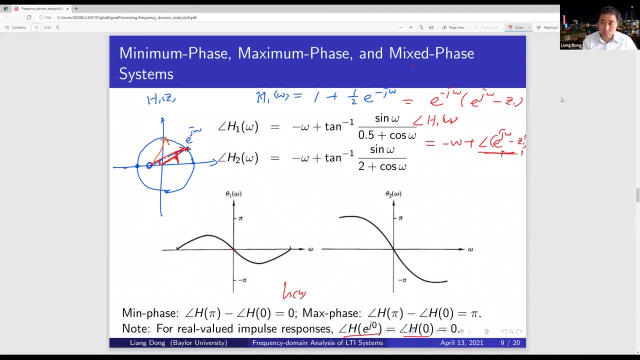 right and it should be somewhere here, Somewhere traveled here, and it gives me a pointing here and to the origin. So this angle is the face. well, actually putting a negative sign here, and that will be in absolute value sense, that will be the largest. 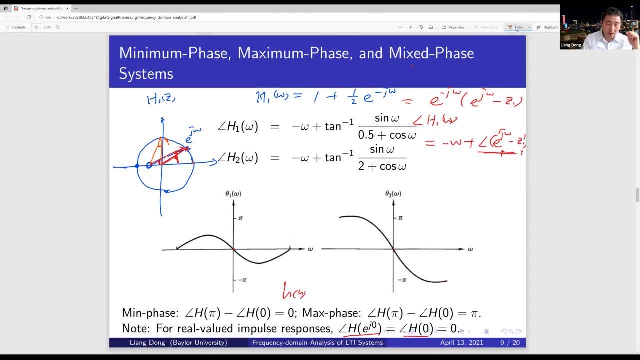 Now, if I, starting from zero, from zero, which is the face angle, is zero, omega equal to zero- then because it deform into a line, therefore this face is zero. right, this angle is zero. If I travel all the way to pi same thing, I got this angle. is you squash that back into zero? So, indeed, we got those. 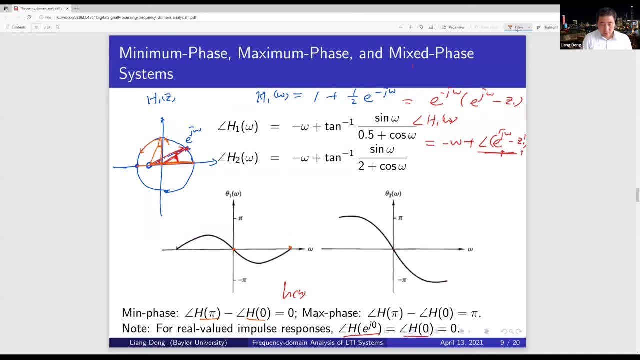 two parts, that is zero and a zero. Now in the middle, when I travel that on a positive, where omega is positive and everything, we have this angle and everything is a negative sign Because we got a negative sign here that's negative omega subtract the angle between E. 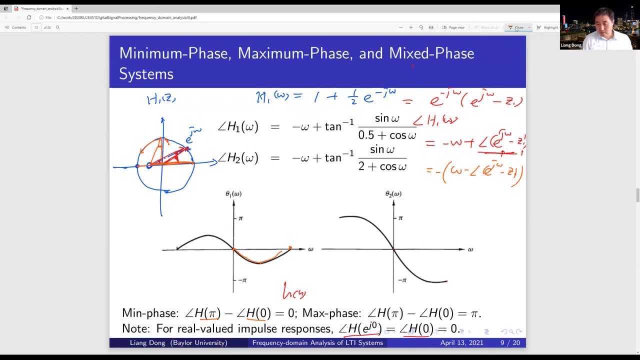 J, omega and Z1.. We got a negative sign here, So that's, everything is negative. Similarly, if I travel on the other side of my of this unit circle, I got a positive result, I got a positive, and then if you go back to negative pi, it will deform. 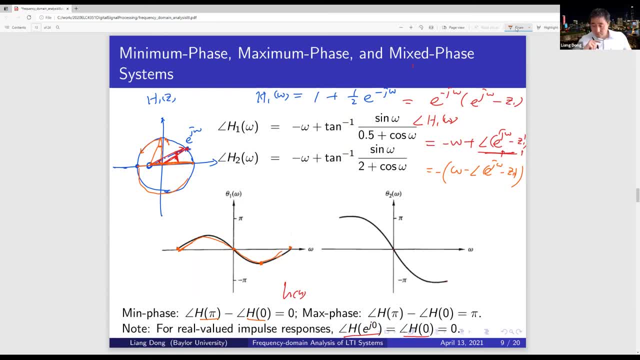 onto zero. so indeed the face should look like that. compare that with h2,. let me very quickly work on the second part for h2, now, if we are looking at the this image here on the z-plane, we have a zero that is outside the unit circle. it's here at the negative two. similarly, 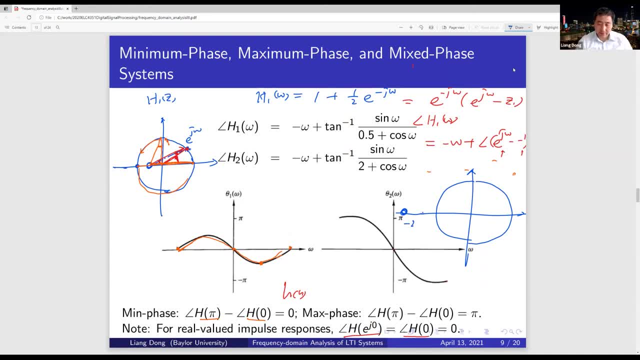 when we calculate the face angle at any point on the unit circle which is e to the power, j, omega, then what we did is we are finding this angle. that's the difference between here and here. so the angle is this angle and of course you take a negative sign. 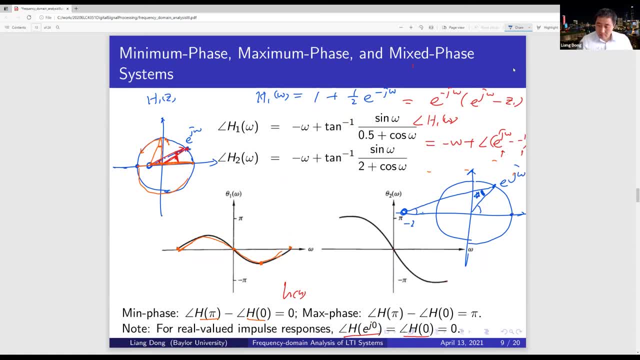 so same thing. if I'm starting from a point here when the face is equal to zero, then this angle is zero. so, starting from zero, when I move on, when I have a positive omega, then I have this angle because it's negative sign. everything is negative. when I travel all the way to here, to pi,